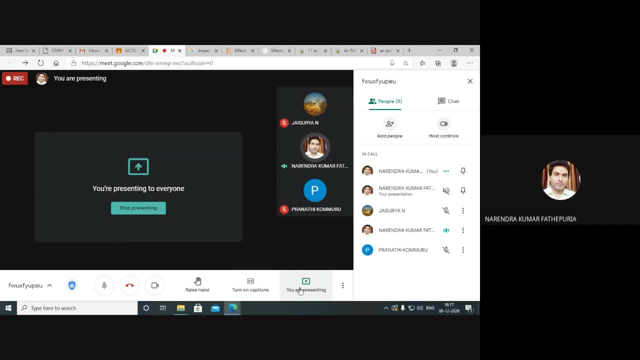 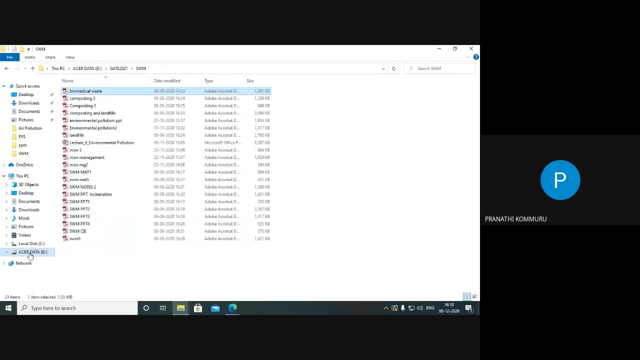 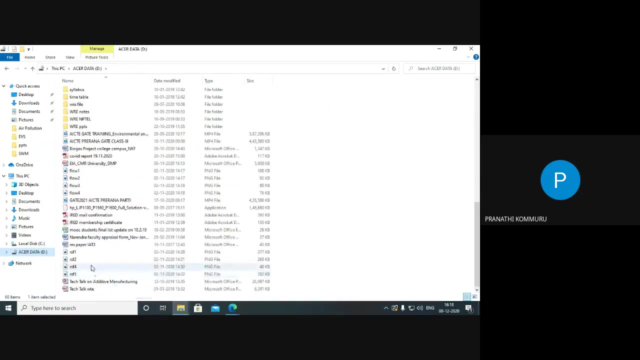 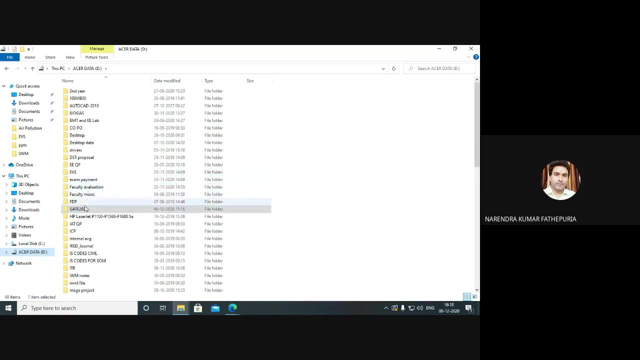 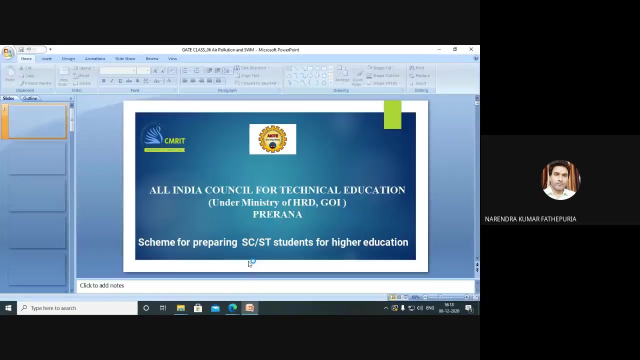 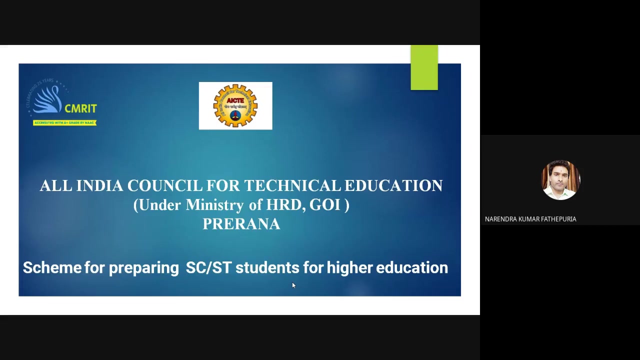 I will try to finish the air pollution. then I will go for the solid waste management part. Is it okay, right? Okay, sir Pranati, is there, Pranati? Yes sir, Yes sir, yeah, so today it's a sixth session, like last session actually. 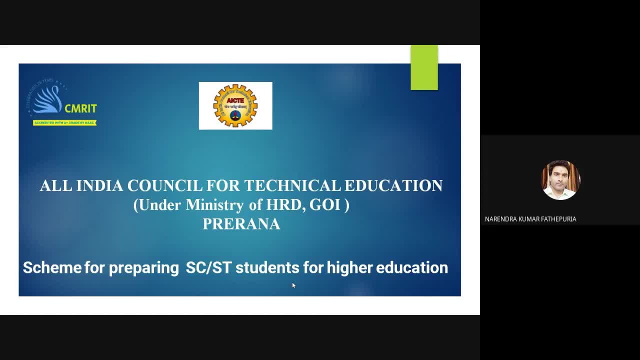 so, professor narendra, here, these are the classes has been recorded for the ICT, parent initiatives for the great aspirants, and this is the first session from CMR technology. so today we will be discussing. we are discussing about the environmental engineering one and two levels for the water and wastewater treatment, water treatment and supply, and 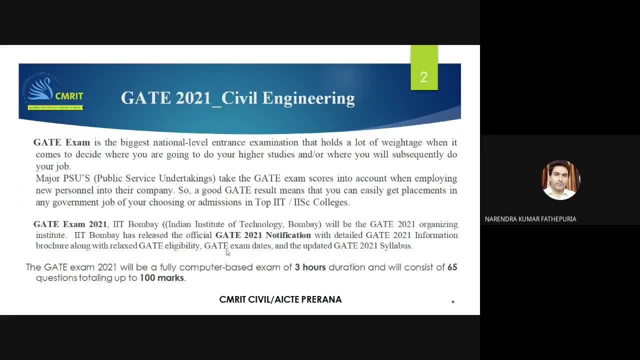 wastewater engineering. this is like we are moving for the next portion, for this is related to air pollution and control management, as well as our solid waste management. there are in the all classes. we have told about the gate to thousands of given fashion, how we'll be on exam pattern will be there and I did bomb. 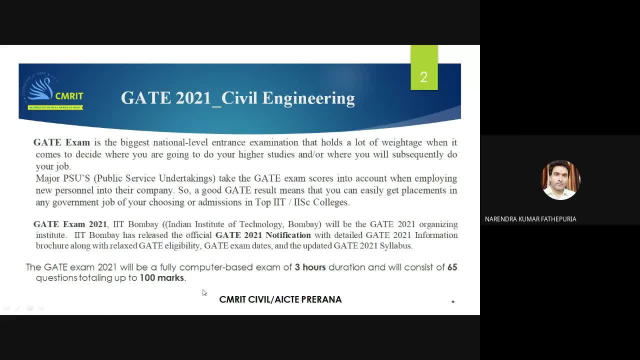 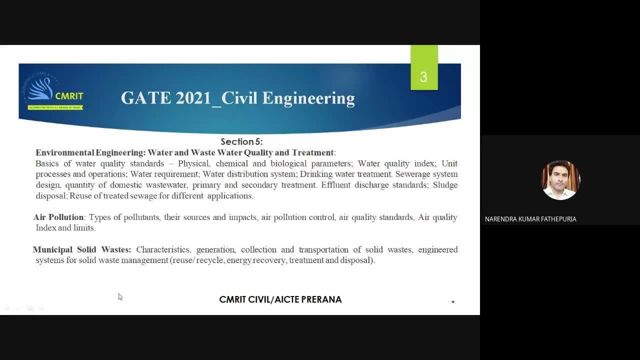 risk and they're detecting this things and there will be a hundred marks, which is right. so this is the portion for the environmental engineering. I'm considering water and wastewater, water quality in treatment part. we have covered it. so we have done everything here and my previous lectures we have 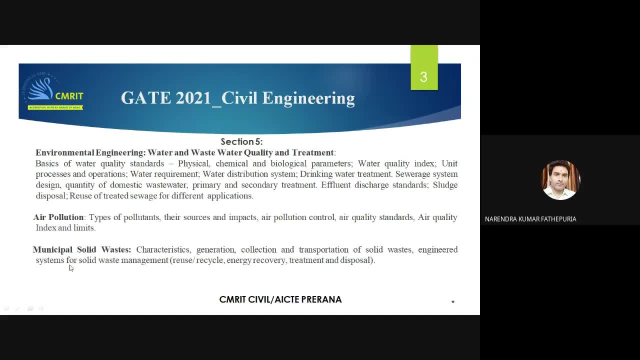 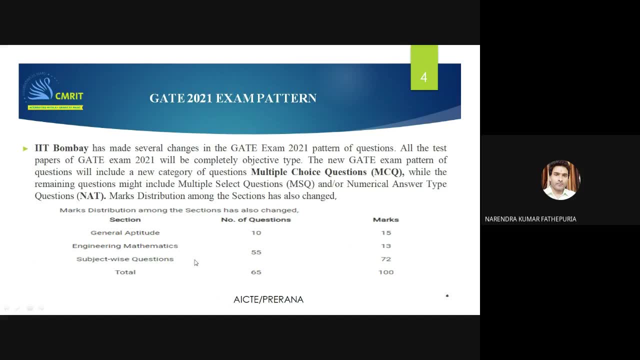 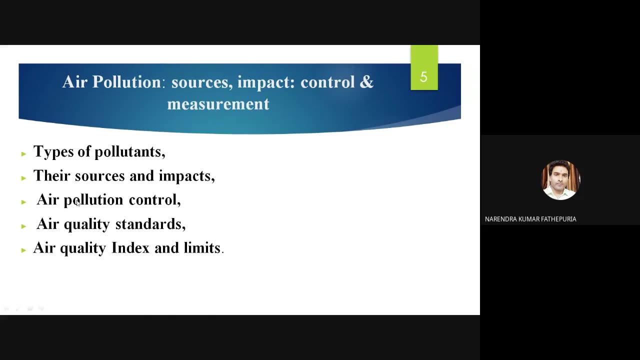 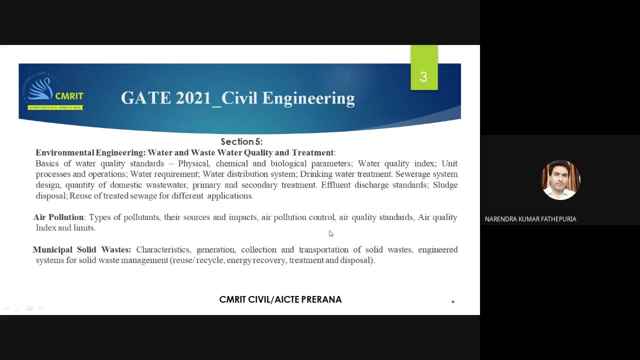 completed this. today I will be discussing about the air pollution as well as the municipal solid waste management. let's just start for today. I will just say that this is just some of the examples. here are just to give you some of the examples of the activities that are there in the area students heading to the air pollution part of the air pollution part: sources, impact control in measurement. we see if you look at this label part, you are concerning about the types of pollution. they're sources in impact, air pollution control, air quality standard and air quality index and limits. so 1-2 marks for this and then 1-2 marks for the Minnesota Validated. so altogether static has been given here. static has been given here. so 1-2 marks for the Minnesota Validated. so altogether static has been given here. 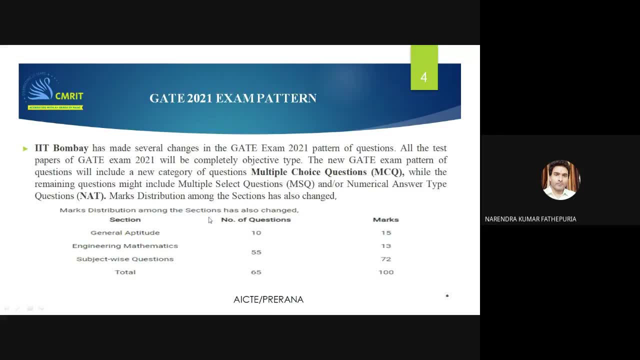 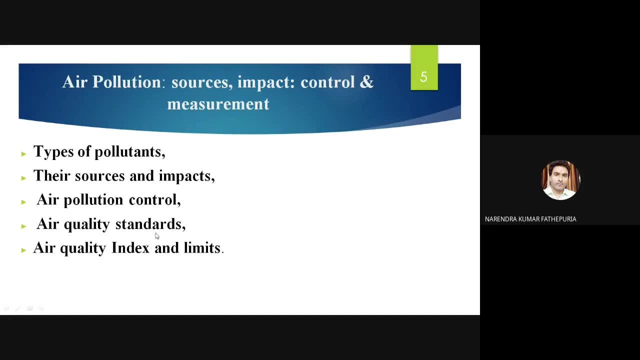 So first you have to understand what is pollution actually and what are the pollutants. Especially we are talking about the air pollution, as actually there are the four types of pollution which are typically noted, which is the water pollution, air pollution, soil and land pollution. 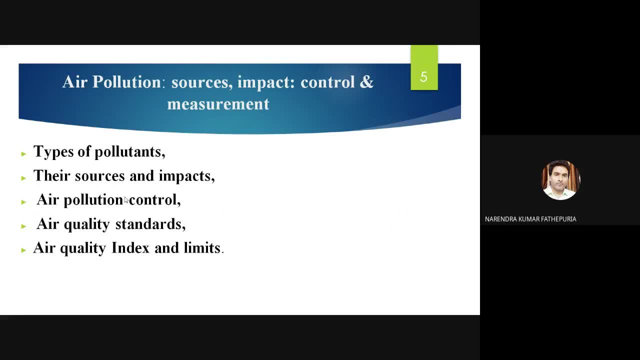 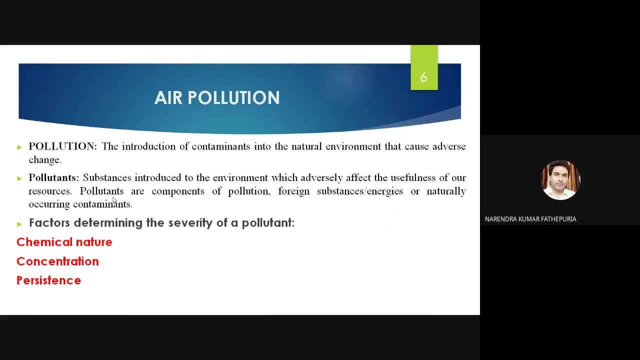 and noise pollution, So anything which is not desirable for the environment, anything which create a problem for the environment, anything which cannot be digested, which cannot be biodegraded, it creates a harmful impact for the ecosystem as well as the living as well as non-biotic system, which is called as pollution, environmental pollution. 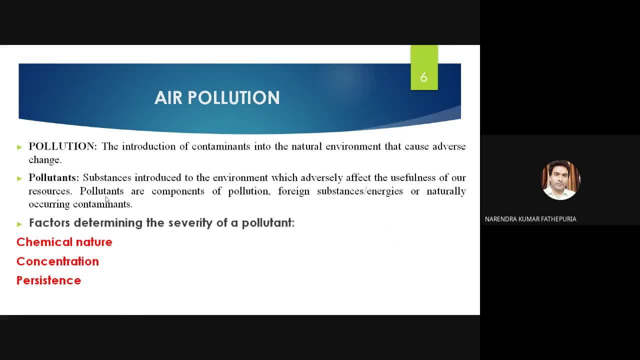 And maybe in terms of water pollutants. if the water pollutants are there causes the water pollution. maybe it is in terms of air pollution. So today we are talking about the air pollution Basic terms: the introduction of contaminants into the natural environment that causes adverse changes. 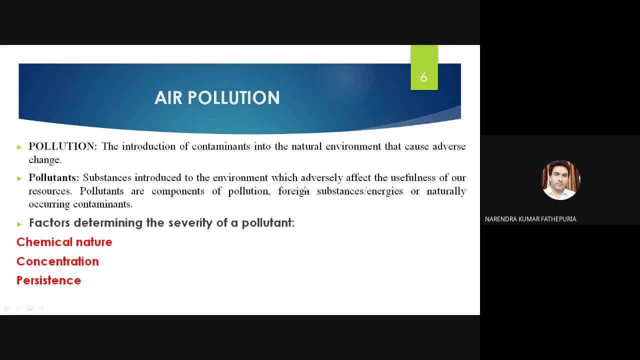 The pollution means substances introduced to the environment which adversely affect the usefulness of our resources. Pollutants are component of pollution: foreign substances, energies or naturally occurring contaminants. Factor affecting the severity of the pollution is the chemical nature, concentration and persistence. These are the three things. 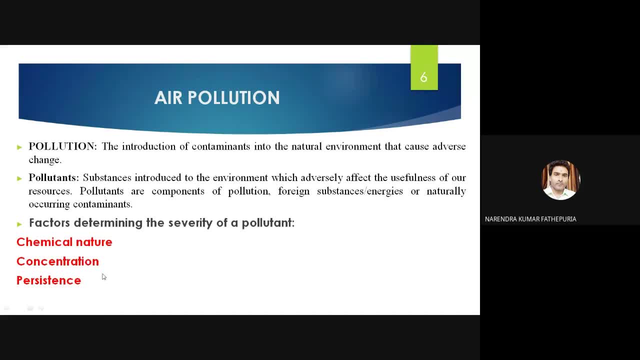 Which has to be noticed in any kind of pollutants. So first the pollution, you have to understand whatever pollution it is. Once you identify you have to go for what are the pollutants are responsible for creating this air pollution? Suppose I am talking about the air pollution- various industries, various automobile vehicle combustion. 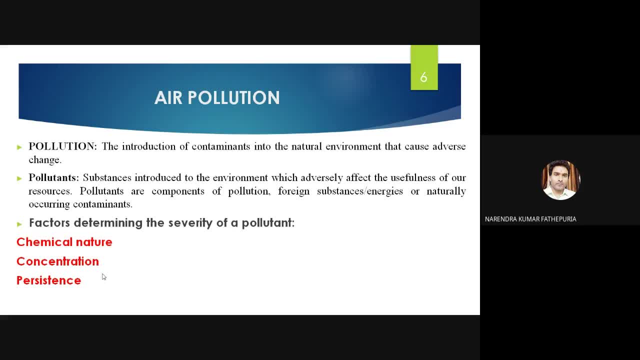 and even the domestic areas. also, there is indoor pollution and outdoor pollution. There is rapid industrialization. there is thermal power plant production unit, automobile industries. There is a cluster of industries- textile, cotton, synthetic textile, paper- import industries. 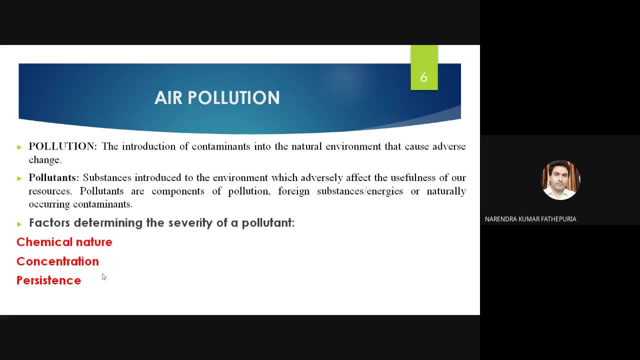 Everywhere, if you see even the steel manufacturing industries, everywhere, if you see there there is a sort of air pollution. they are generating it through the state. They are burning something on a very high temperature. they need energy. In most of the cases they are. 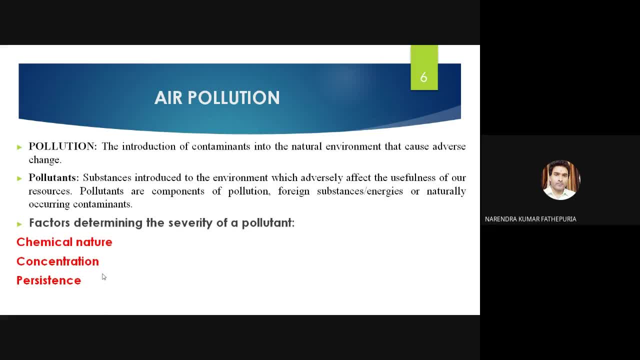 Fossil fuel based energy emission is going on. So if you are burning a fossil fuel, of course the various types of pollutants will be releasing into the atmosphere. So the three things are important. One is the chemical nature. You have to understand the pollutant chemical nature. 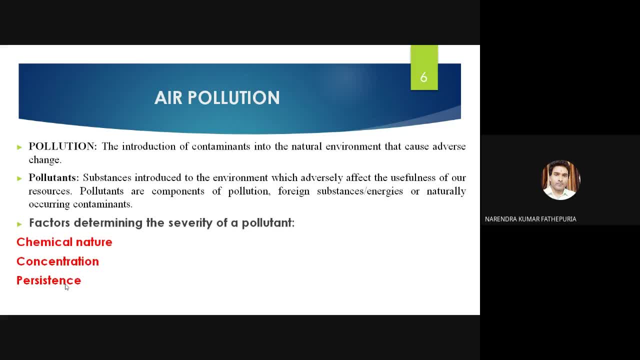 Second one is the chemical nature means how it is reacting with the original composition of the gases, right? So we have in, If you see the atmosphere- I will talk about the atmosphere, right- Various layers and all that, And we have a typical composition of the gases. 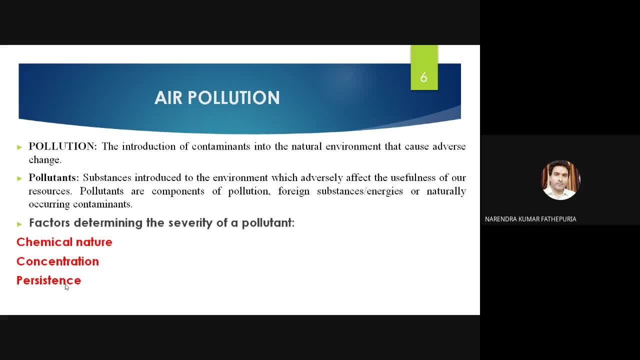 So once this pollutant is released into the atmosphere from the various types of sources, So what is How it is chemically react with the existing gases, How it is react chemically with the existing environment And what is the composition? finally, 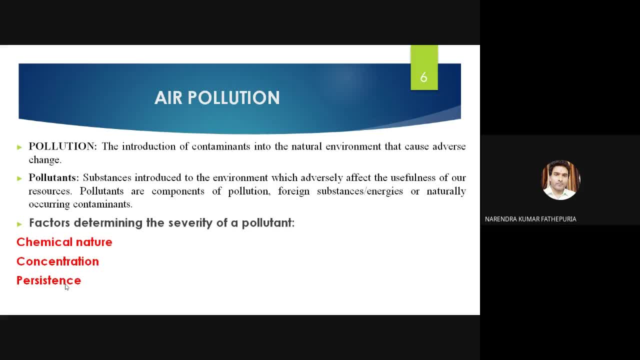 Once the chemical reaction is completed, what is the further- We can say the chemical acids, whatever the component, toxic compounds will be generated And how it is harmful for the environment. Second, is the concentration? On what concentration, What percentage it is diluting? 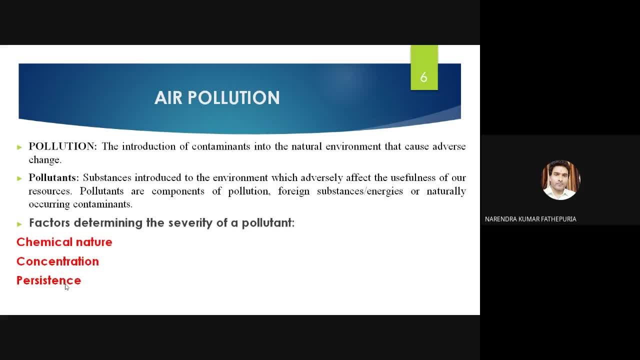 What percentage it is dispersing, What percentage it is, We can say the mixing with the environmental gases. That is important. So concentration you have to identify. So for that there is a measurement technique. Once you identify the pollutant, you have to measure the pollutant. 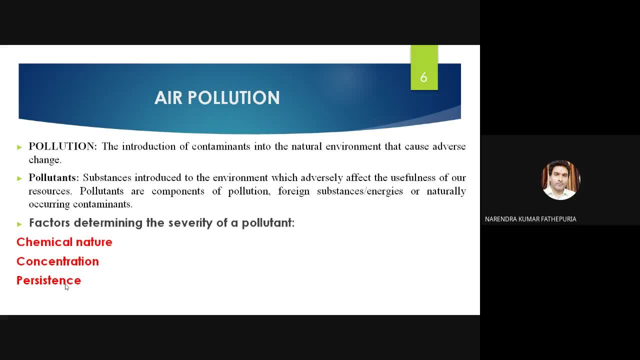 There is the various air pollution measurement devices: Air sampler, analyzer, volume samplers, And then we have a. We have a NOx samplers for capturing the particulate matter, for the concentration We have a particulate matter, PM10 and PM2.5. 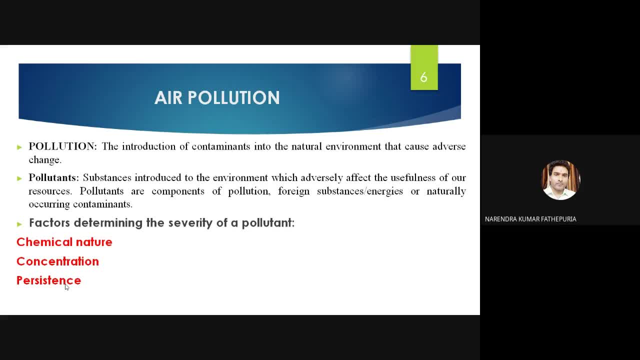 So various pollutant measurement devices we have, We have to check the concentration in the air first, Then we can understand, we can tell the severity of the condition for the particular type of pollutant And we Of course these pollutants are having bad impact on human beings everywhere. 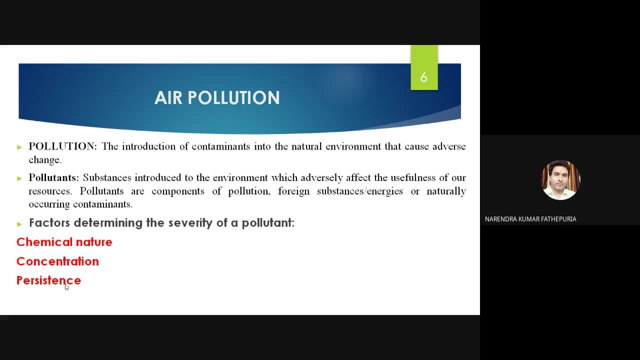 Right, I will be talking about the impact of these air pollutants in the atmosphere, Right And second. third one is the persistence in nature The pollutants which How long it will sustain into the atmosphere, How long it will survive, Right. 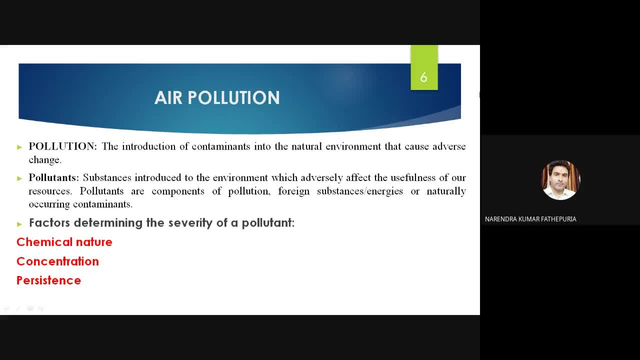 If it is not decomposed, if it is not biodegraded in the nature, For how long it will survive? How long it will be there in the nature, Maybe in a dilution form, maybe in a persistent, maybe in a dispersant form? 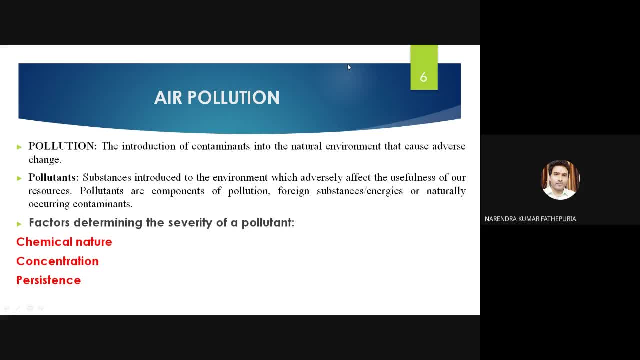 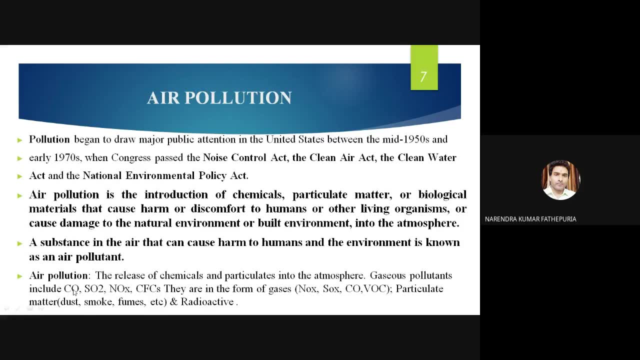 Or maybe it will mix with the water, Right? So these three things has to be measured before going for any kind of pollution. So today I am talking about the air pollution part. So pollution terms begin to draw major public attention from the United States between the mid-1950s and early 1970s. 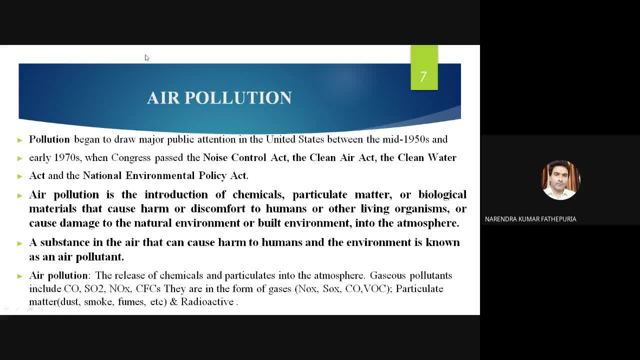 Then the Congress passed the Noise Pollution Control Act and then Clean Air Act, as well as the Clean Water Act. The National Environmental Protection Agency, The National Environmental Policy Act, has also come. There is a US EPA Environmental Protection Agency which has formed these laws. 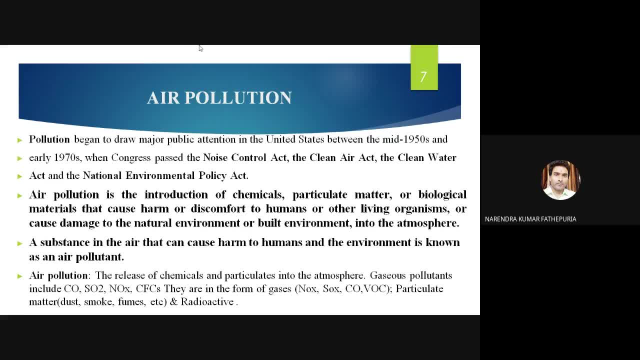 Right. So what is the air pollution exactly? You see that The air pollution is the introduction of chemical particulate matter or biological matters- materials that cause harm or discompose to human or other living organisms or causes damage to the natural environment or built environment- into the atmosphere. 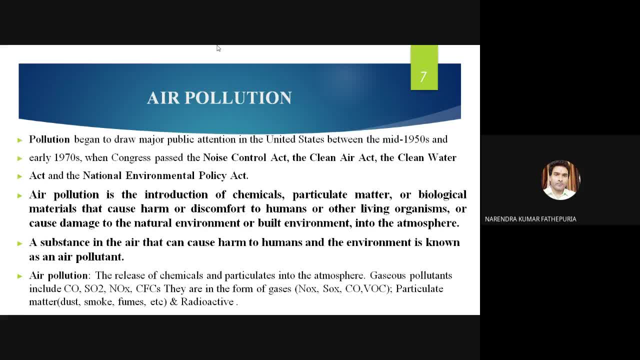 A substance in the air that can cause damage. A substance in the air that can cause harm to human or environment is known as an air pollutant. These are the well-known air pollutants. We have a classification of the pollutants. There is a primary air pollutant as well as the secondary air pollutant. 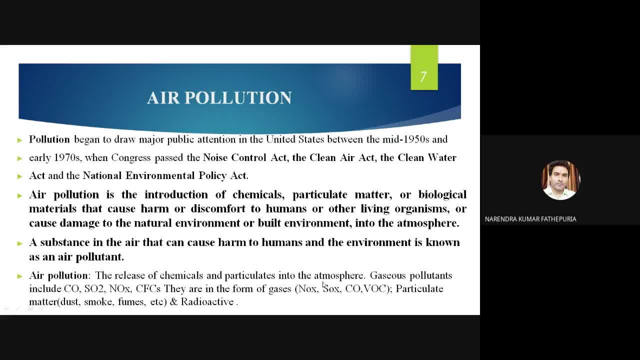 So commonly we have seen the release of chemicals and particulates into the atmosphere. The gases pollutants include carbon monoxide, sulfur dioxide, the various forms of sulfur, and then NOx, nitrogen dioxide, NOx, NO2 or NO3.. 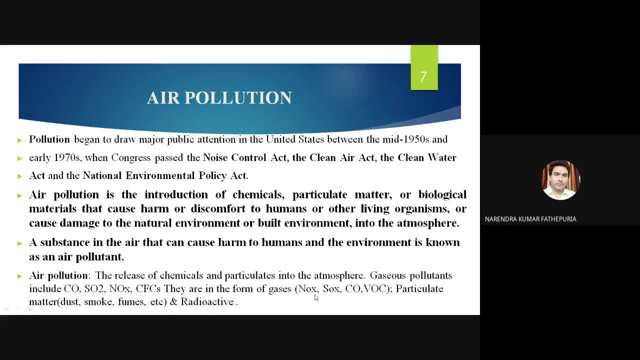 Then chlorofluorocarbons. They are in the form of various gases: NOx, SOx, carbon monoxide, volatile organic compounds, particulate matters, dust, smoke, fumes, mist, and there are particulate matter PN2.5, PN10,. 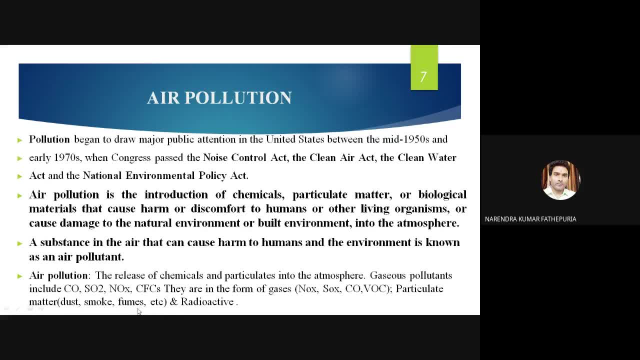 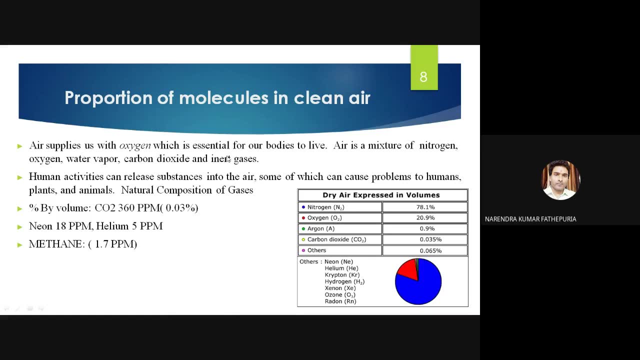 which are responsible for the air pollution. Right, The smoke is also one of one type of pollution only. And then various radioactive gases which will also release into the atmosphere, causes the air pollution. So we see the first carbon, So we see the first composition of gases in a clean air, in our atmosphere. 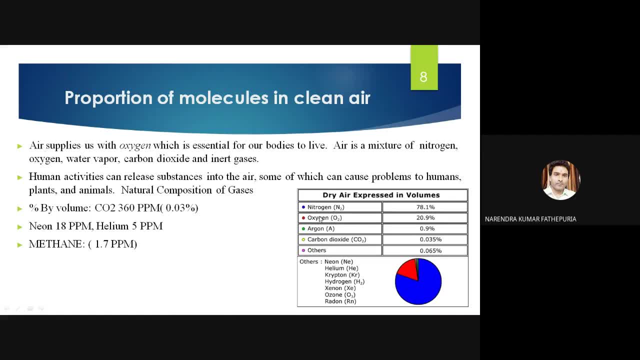 There are the. this is the typical composition of gases. So, without any pollution- These- this is our atmosphere- We have a typical composition of these gases, right? So nitrogen is roughly 78.1%, Oxygen is 20.9%. 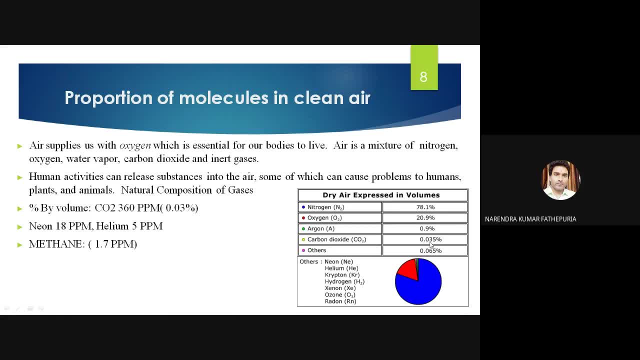 Argan is 0.9%, Carbon dioxide is roughly 0.035% And other gases are 0.065%, And some of the other inert gases are also there, like neon, helium, krypton, hydrogen, xenon, ozone, radon, right. 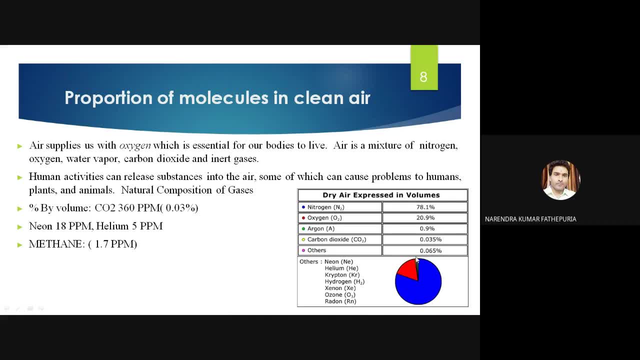 So this is the pie chart. If you see that we have a 78% or 79% of nitrogen, only The remaining 21%, 20.9, 21% is the oxygen. This is the percentage weight by volume. 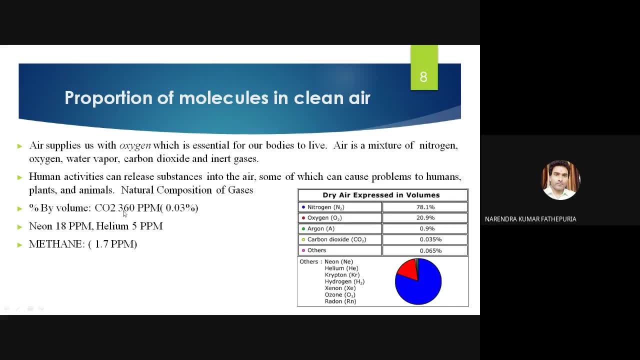 So CO2, carbon dioxide, is around 360 ppm. They are 0.03% for the total. Neon is 18 ppm, Helium is 5 ppm And methane is 1.7 ppm roughly. So these are the typical fresh composition of gases in our atmosphere. 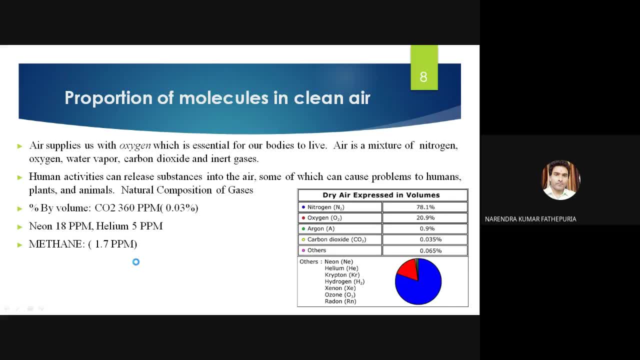 Now, once the pollutant release, these types of pollutant release, and it will mix with the atmosphere, it will react with these gases and it will form various through the various chemical reactions and various biochemical reactions will be taking place And they will react. 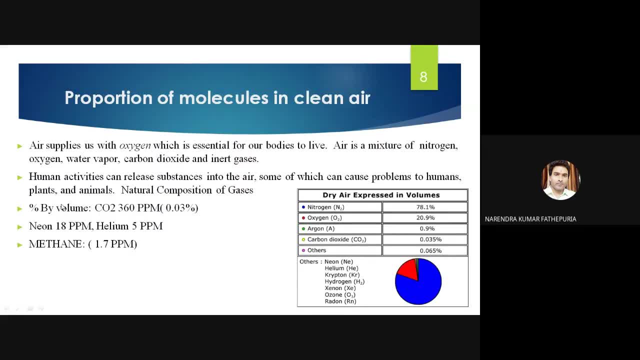 They will form the pollutants right. Secondly, pollutants and all that, So human activities, can release substances into the air, some of which can cause problems to human plants and animals. So there is an impact on human impact on plants as well as the animals. 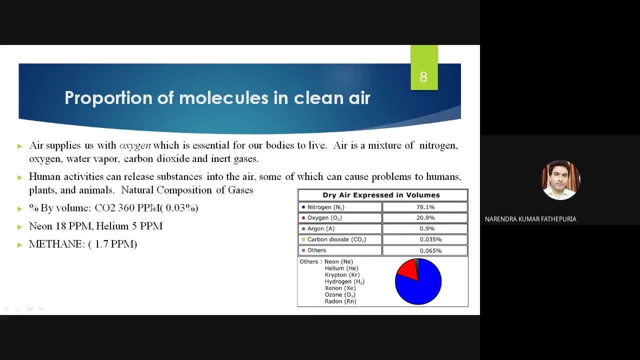 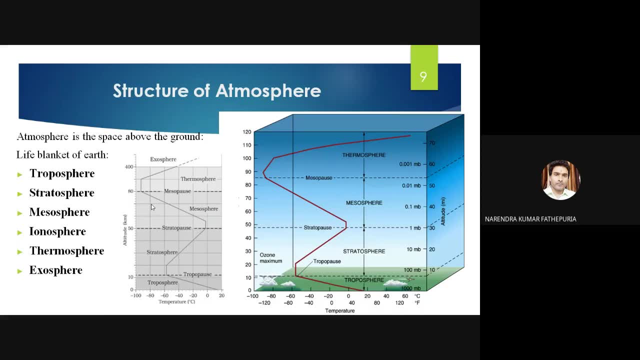 There is a natural composition of gases. we have explained. now, right, We will go for the control and measurement technique. then we will talk in detail. This is the structure of the atmosphere. This is our atmosphere above the earth. This is the structure of the atmosphere. 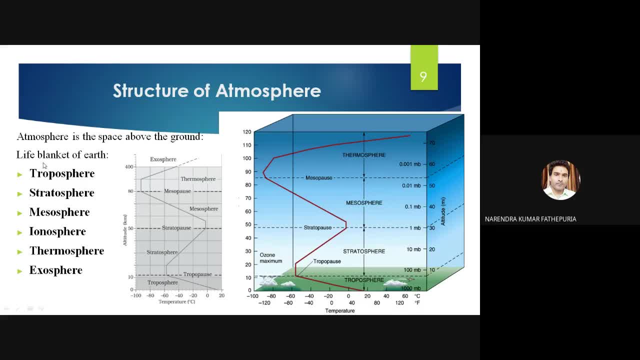 So atmosphere is the space above the ground And this is the life blanket of earth. These are the various spheres that we have. we have divided our sphere above the ground. We have divided our sphere in various forms, So there is a tryposphere on the bottom, starting from the ground level to up. 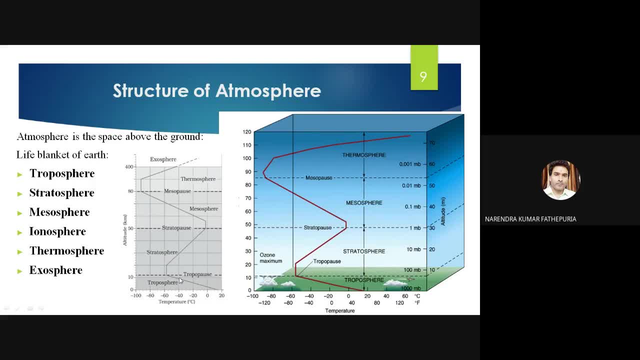 There is a tryposphere layer 0 to 10.. There is a trypopause also. This is a part of tryposphere only. Then second is the stratosphere. After stratosphere we have a mesosphere. 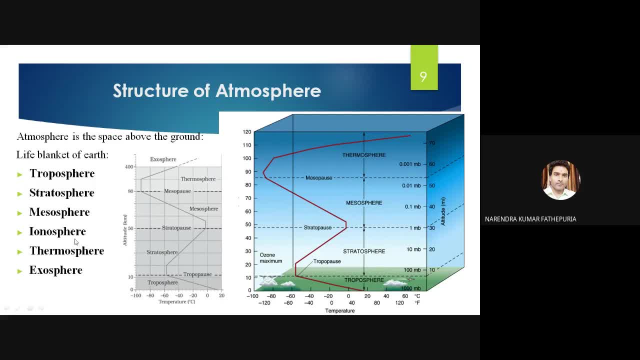 We have a mesosphere, And then we have ionosphere, And there is a thermosphere And there is a exosphere, right. So various conditions regarding the temperature, regarding the altitude, like height, right Height from the ground. 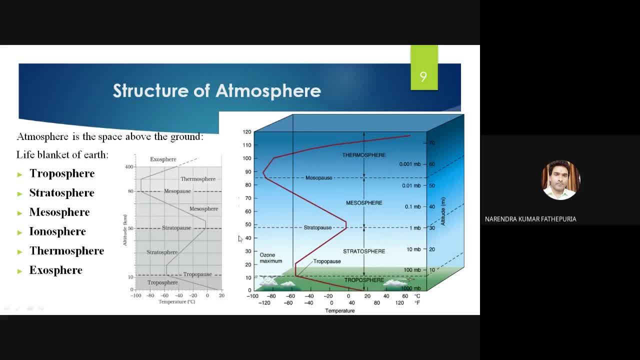 We have divided our atmosphere And there is some gases composition, like the various. the temperature will be different in all layers in all spheres, Like different different temperature in various spheres, As well as the pressure will be different. Wind direction and wind speed also will differ. 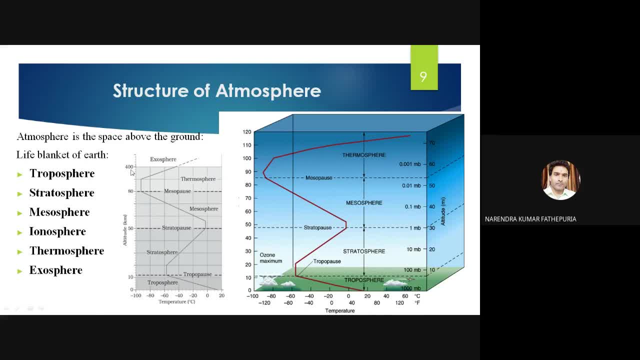 And, respectively, altitude is increasing, The temperature is also decreasing. So, like this, there is a lot of climatic factors, meteorological factors that will play an important role, And so we have divided our whole atmosphere in three or six spheres, actually. 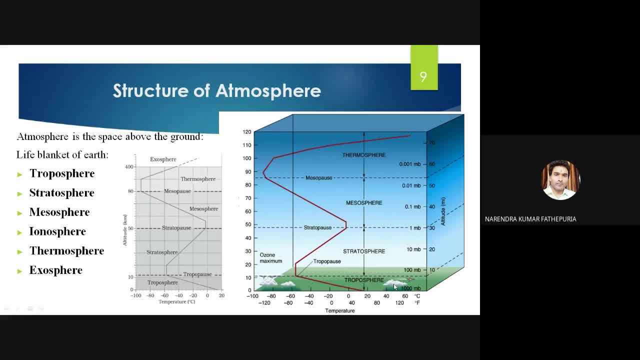 Tryposphere, stratosphere, mesosphere, ionosphere And thermosphere, exosphere. This is the distance given, And then various gases. composition also, we have explained here. This is the altitude And this is the temperature. Temperature- how, what is the temperature? and various spheres. 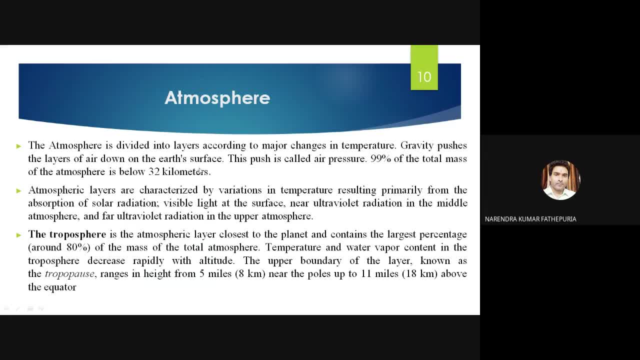 Okay, Yeah, So atmosphere is divided in layers according to the major changes in temperature. Gravity. possess the layer of air down on the earth's surface. This process is called as air pressure. 99% of the total mass is air. 99% of the total mass of the atmosphere is below 32 km only. 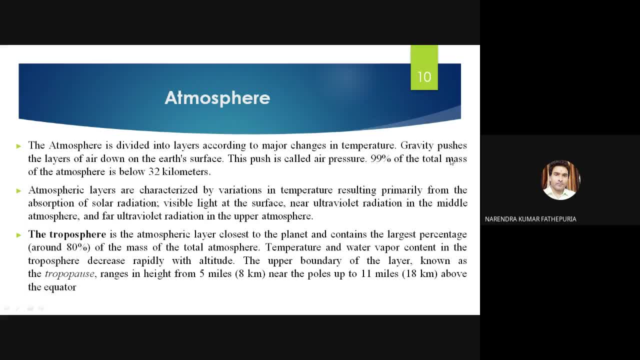 This is all this is we have noted down. 99% of the total mass of the atmosphere is below 32 km. Our atmosphere layers are characterized by variations in the temperature resulting primarily from the absorption of solar radiation Visible lights at the surface. 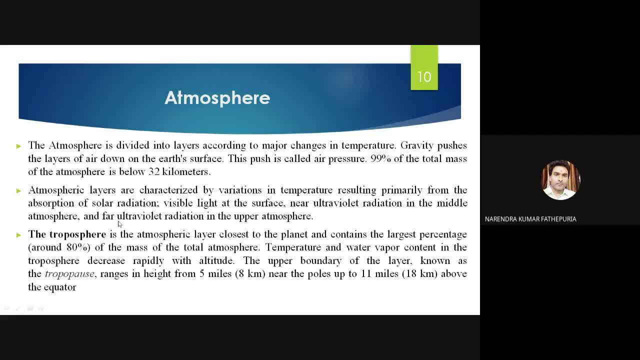 Near ultraviolet radiations in the middle atmosphere And the far ultraviolet radiations into the upper atmosphere. UV radiations play a very important role because it's a harmful wave which are getting a lot of problems. So that's why the ozone layer protect from the UV radiations. 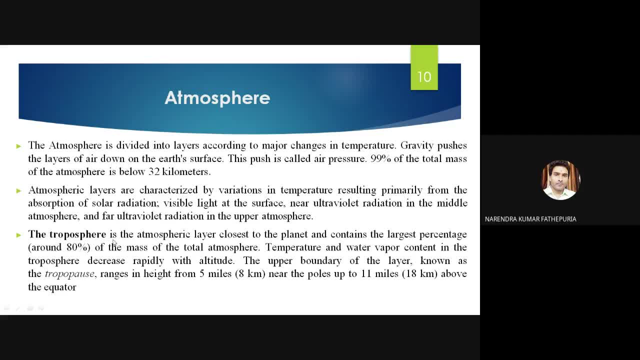 So these are roughly things that you already know about it. There is a troposphere, So we'll talk, start from the troposphere, This one. If the atmospheric layer closes to the planet and contains the largest percentage- around 80% of the mass of the total atmosphere. 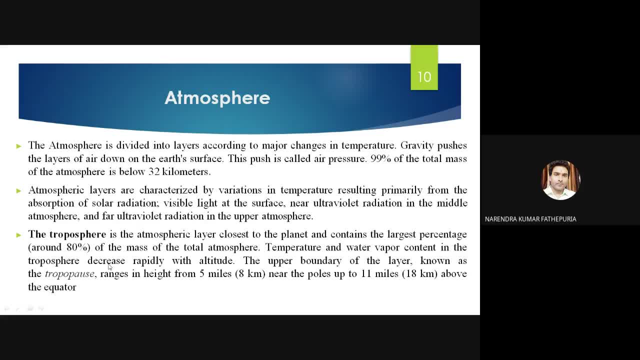 Temperature and water purpose contains in the troposphere Decreases rapidly with altitude. The upper boundary of the layer known as the tropopause ranges in height from 5 miles, or 8 km, near the poles, up to the 11 miles, or 18 km, above the equator. 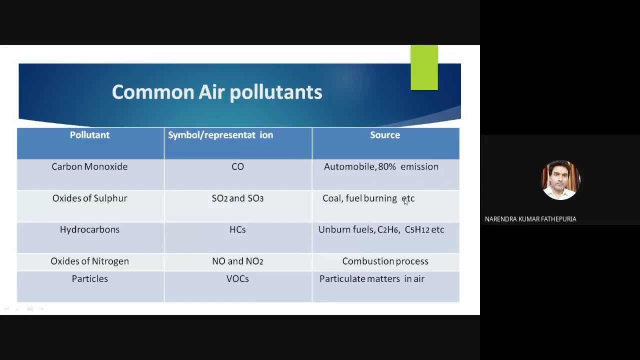 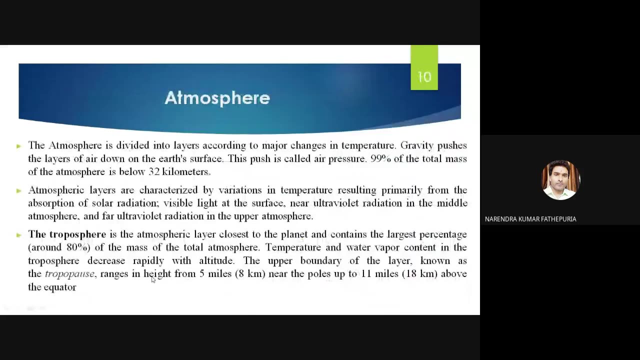 Now we'll come for the pollution. These are the common air pollutants which are responsible. I have here also have briefly told about the pollutants. Okay, Now I will go for the classification sources As well as the representing symbols. Right, 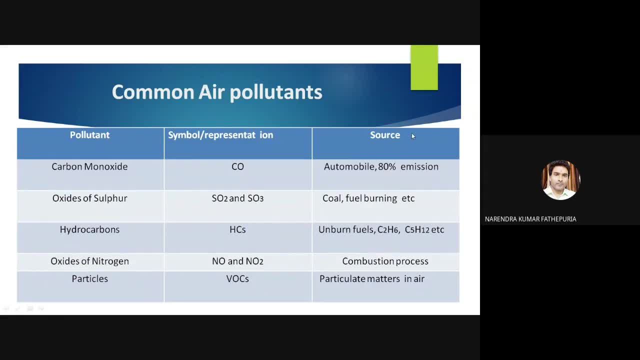 This is the carbon monoxide. Carbon dioxide. also, Most of the 80% it will come from the automobile emissions, As well as the fossil fuel based industries, also Where the incineration and burning is happening. Various oxides of sulfur. 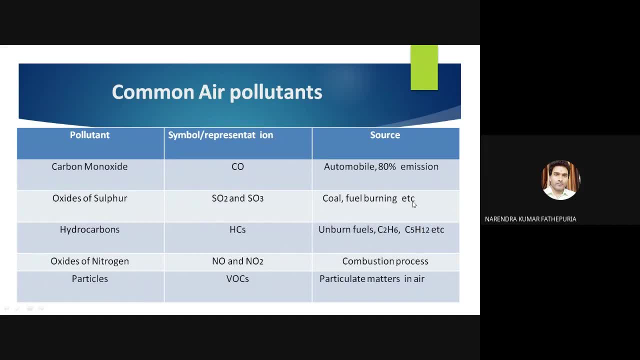 SO2 and SOx, SO3 and SO2.. Coal fuel burning, etc. There are the hydrocarbons also. Hydrocarbons, Unburned fuel, C2H2.. Various benzene formation and all that Carbons will be releasing again from the industries and unburned fossil fuel emissions automobile vehicles. 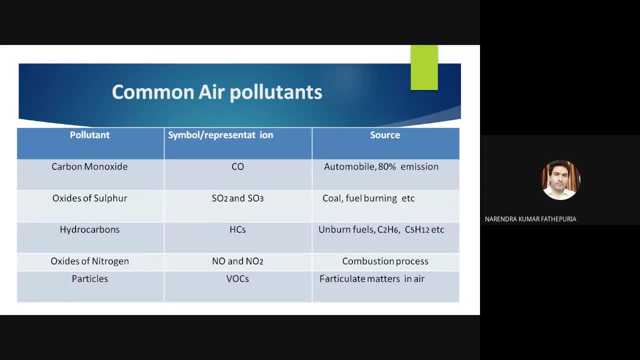 100% combustion will not happen inside the internal combustion engine, So unburned fuel, Releasing this hydro, releases this hydrocarbons, Which will create a lot of problems for the as the main reason for the air pollution. actually, 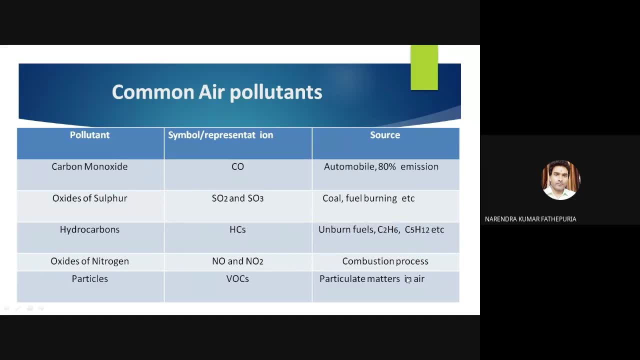 Various oxides of nitrogen, NO and NOx and NO2.. Combustion process: it will release And particulate metals like volatile organic compound, PM2 and PM2.5 and PM10. And suspended particulate metal, also Respiratory suspended particulate metal. 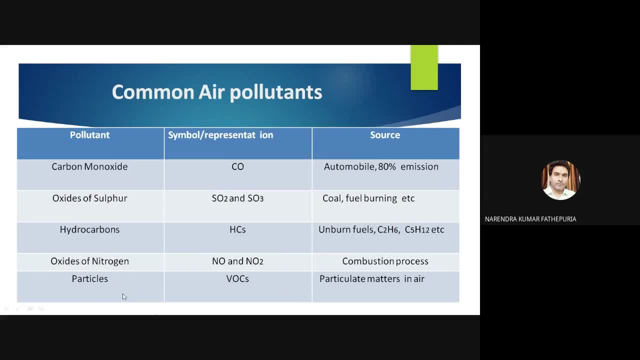 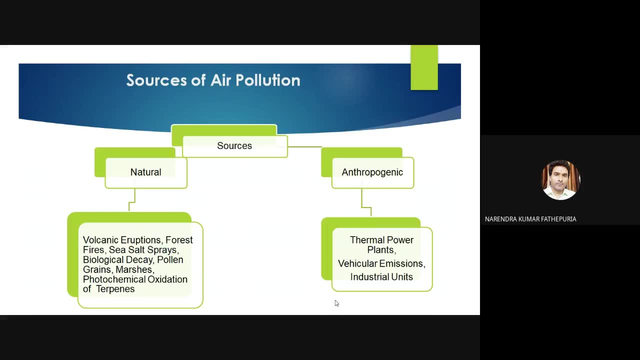 We will go for the again. classification for the particulate metals and particles: Okay, Maybe it will be in suspension and dispersion form: Suspension in most of the cases. These are the sources of air pollution. There are the two types of sources of air pollution. 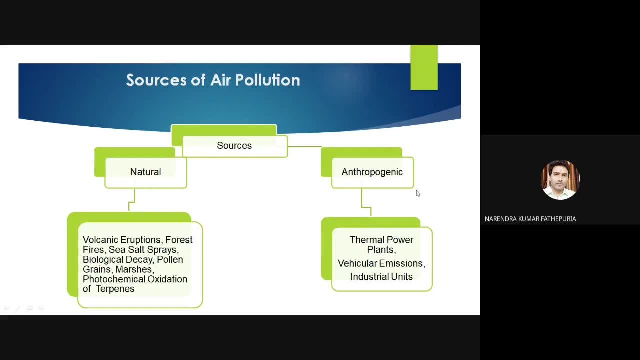 One is the natural resources, Another one is the anthropogenic regions. Anthropogenic regions means the man-made regions That man has created this pollution. So if you see the natural resources of pollution We have, like forest fire, volcano eruptions, sea salt sprays, biological decays, pollen, grains- 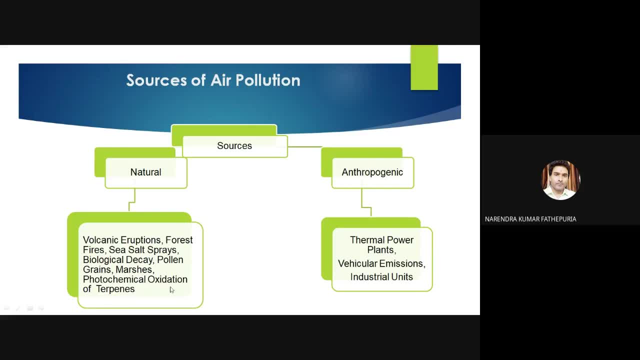 Masses. Autochemical oxidation of terpenes causes the natural sources of pollution: Thermal thunderstorms, sometimes So in volcano eruptions. These are the main reasons for the air pollution. Natural reasons: These are associated with the man-made region actually. 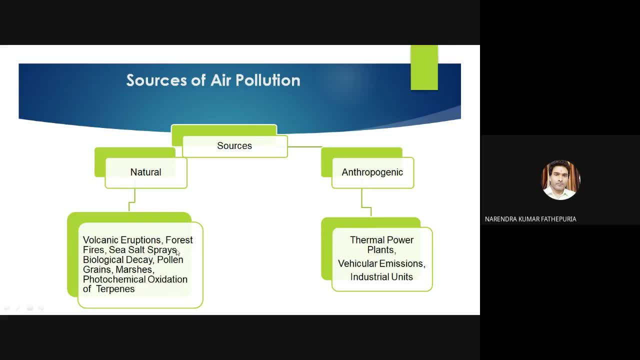 Because of the forest fire and these all the regions are coming again Because of the excess mining as well as the cutting the forest Deforestation happening with the rapid states Right And there is water pollution everywhere, There is air pollution, Soil is contaminated. 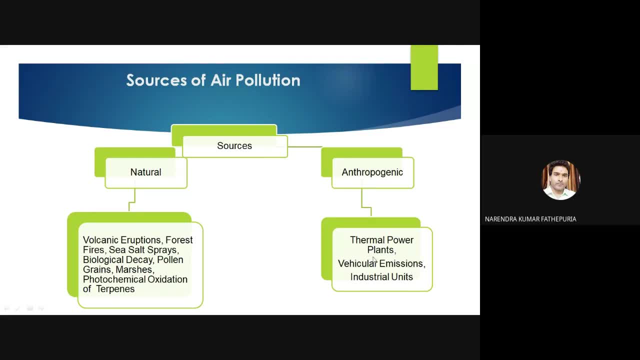 Because of the man-made region. Anthropogenic regions like thermal power plant, Vehicle emissions, Automobile vehicle emissions And various industries are responsible for creating this air pollution, And even the indoor air pollution is also considered nowadays. This is also because of the man-made regions only. 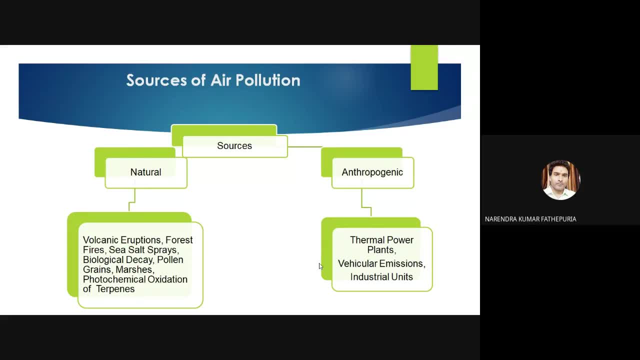 Excess, population rise and rapid urbanization is also the main reason for the air pollution And meaningless consumption of the resources, Natural resources, Maybe water, air, soil and whatever The other minerals That we are using it without thinking about it. 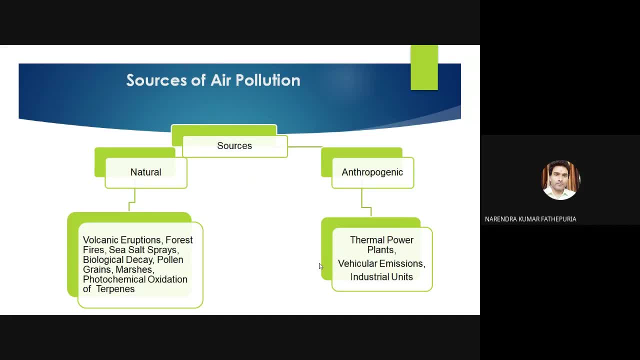 And we are creating a lot of solid waste problem also, And we are polluting soil, We are polluting water, We are polluting air. Most of the reasons are anthropogenic reasons. Excess deforestation is also the main reason we are cutting the forest for the daily needs. 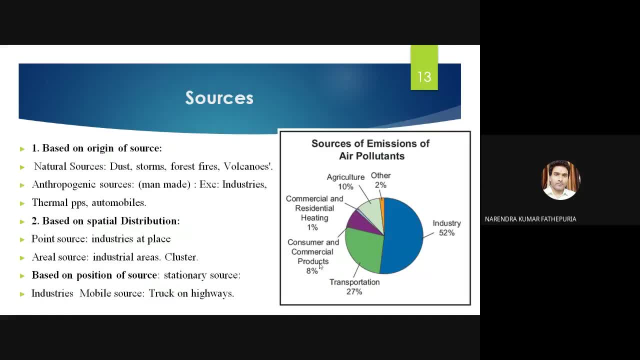 Okay, Okay, So based on the sources has been classified here. These are the sources of emission of air pollution. What is the percentage that is causing the air pollution? So industries contribution for this air pollution is 52%. Various types of industries. 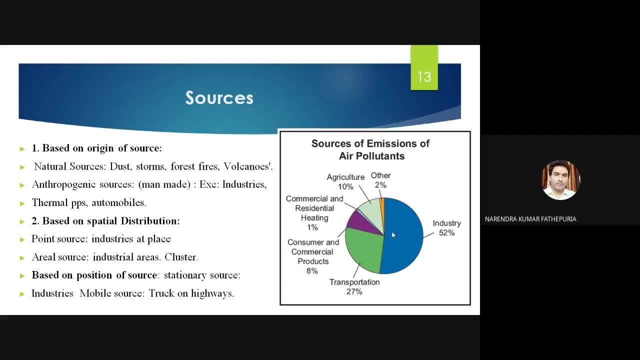 Automobile production, manufacturing, textile, steel manufacturing, thermal power plants, Cotton industry, Pharmaceuticals, Your paper and pulp industries, Daily food processing industries, Cool consumable, EPSI, ENG industries, So all kinds of industries. There is a cluster of industries. 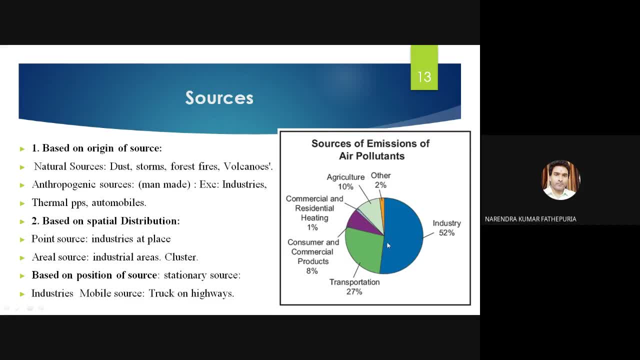 Everywhere we are using resources, Everywhere you are using energy resources and water resources and everywhere. And then you are. there are the big furnaces, boilers, steamers, right, All big machineries are running because of electricity and all that. 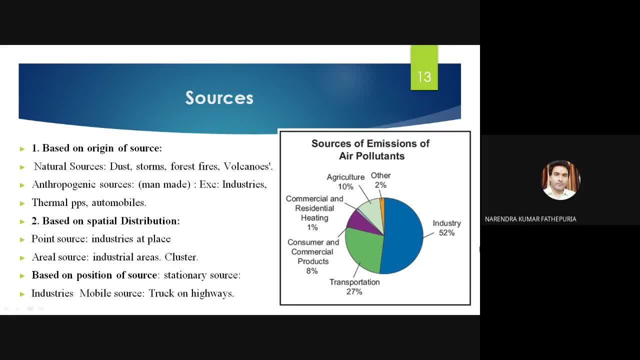 They are using electricity and all that. So everywhere in the world, So everywhere in the form of direct, clean and direct form, they are releasing various air pollutions daily basis. So 52% largest contribution in the air pollution comes from the industry. 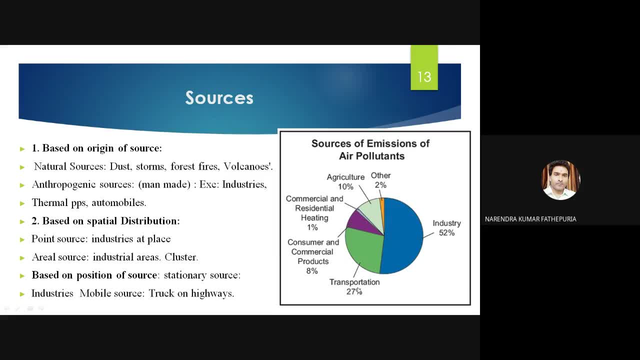 Then from transportation, all kinds of transportation- rail transport, air transport, road transport- all together contributing in this air pollution 27% because air traffic, air transport, also all the aircraft fuel combustion- This is where we are using Aircraft- is using high octane number gas. 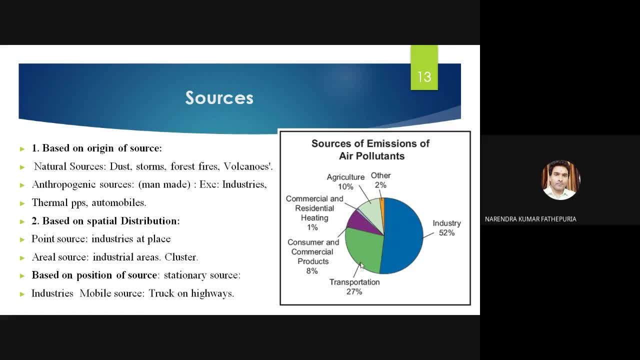 Again creating pollution. All the aircraft carrier, also the satellite carriers, also causing the air pollution. So all together 27% coming from the transport sector. Then the consumer and commercial product: 8%. commercial and residential heating: 1%. Agriculture sector is also causing air pollution. 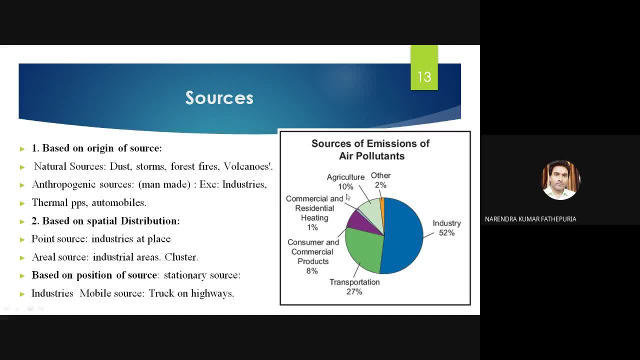 They are going to hold open burning, They are burning their residues at the farm, Then again creating air pollution. All together 10% and remaining 2%. So sources are there. So sources has been classified herein, based on the origin of the source, based on the 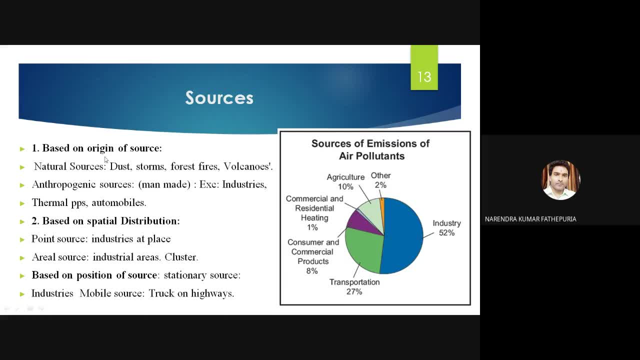 spatial distribution. The number first is based on the origin of the source. We have a natural sources like dust, storm, forest fires, volcano eruptions. anthropogenic sources like manmade exos, industry, thermal power plant and automobile. We have classified the origin of the source. 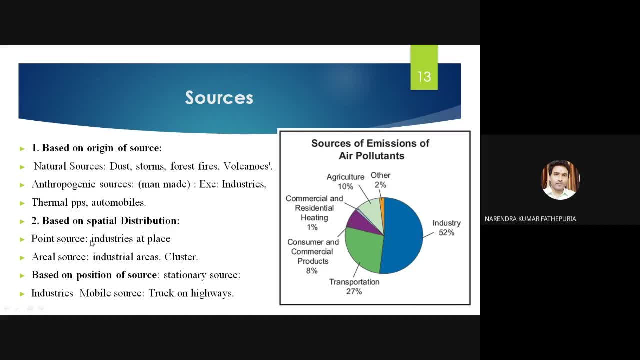 Second, is based on the spatial distribution. We have a point source based on the spatial distribution, Point source, like industry, So the industry is at place. There is a movable source as well as the fixed source, also based on the position, Like the aerial sources, like industries, industrial areas and cluster of the industries are causing. 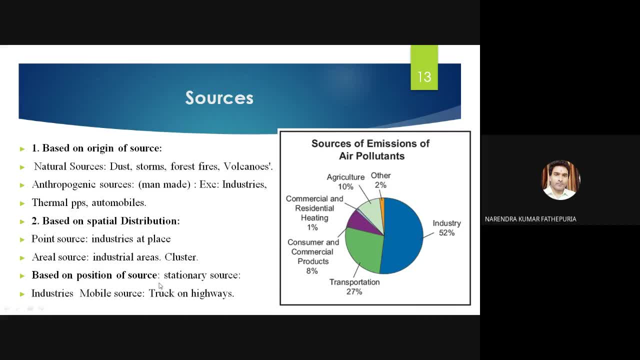 the pollution And then based on the position of source. also, there is a stationary source of pollution and there is a movable source of pollution. The stationary sources are, like various industries, which has been fixed on a particular location and creating a pollution, generating a pollution day by day. 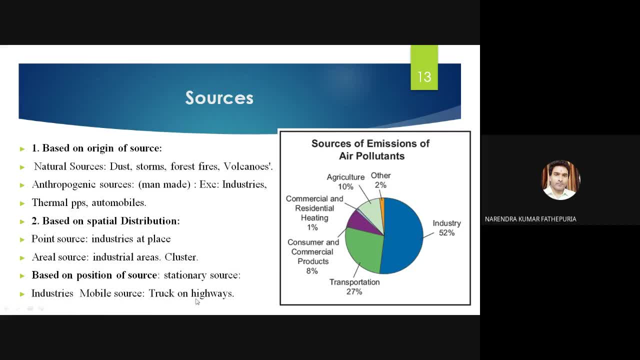 Then there is a movable source like the truck on highways movable source. Then there is a stationary source like the aircraft carrier. Then there is a movable source like the highways movable source like trains right. automobile vehicles, aircraft right. These are the movable sources of pollution which is spreading a pollution into that much. 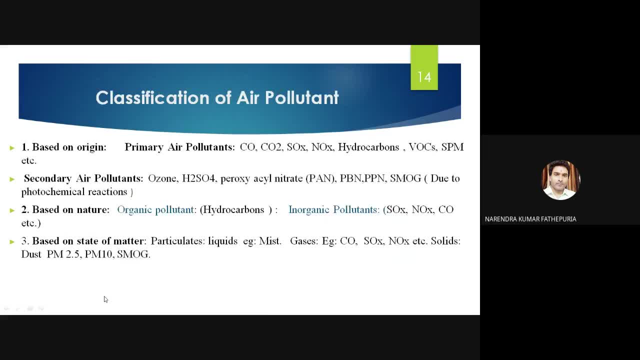 air. Okay. So like this, we have various classifications. Now, based on the origin, we have a primary air pollutant as well as a secondary air pollutant. This is very important: Primary air pollutant as well as the secondary air pollutant. 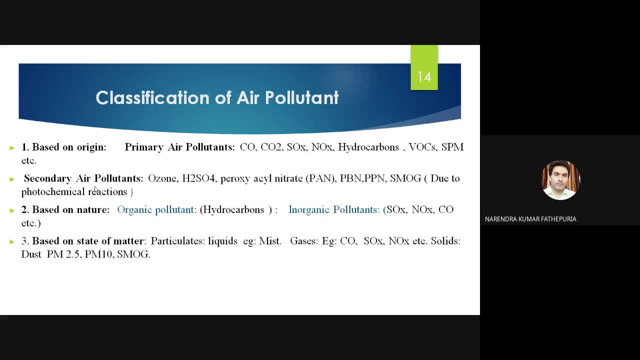 So primary air pollutant which will release directly from the source. okay, like the carbon monoxide, carbon dioxide, various SOx, NOx, nitrogen dioxide and all that, And then various hydrocarbons, Unburnt combustion is happening in fossil fuel based emissions. fossil fuel based combustion. 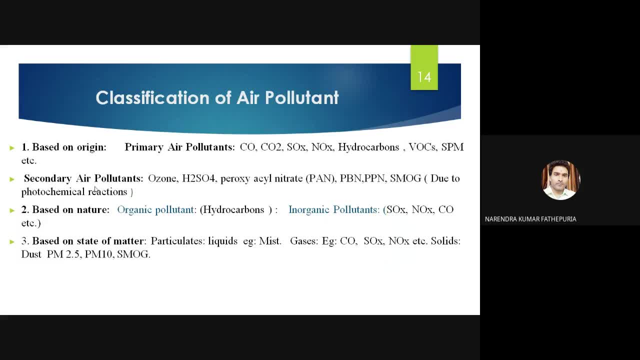 engine internal combustion engines, And then these, the complex chain of hydrocarbons, carbon and as well as the hydrogen these molecules will be coming from the source, And then various volatile organic compounds, So types of hydrocarbons only, And suspended particulate matter also a part of primary air pollutant right. 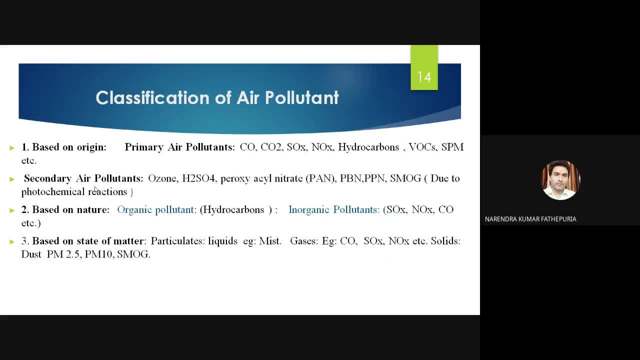 There is a secondary air pollutant. Once the primary pollutants will release into the atmosphere, it will recreate with the atmospheric gases and then it will form the secondary pollutant. These are the secondary air pollutants, Like the ozone, H2SO4, peroxyl silane nitrate. 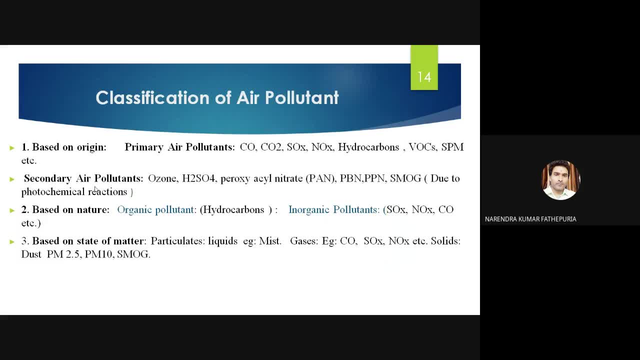 Okay, PN right, H2SO4, ozone, PEN, PBN, PPN, smoke right. Due to the photochemical reactions the smoke is generated. These are the secondary pollutants And based on the nature also, we have pollutants like two types of pollutants. 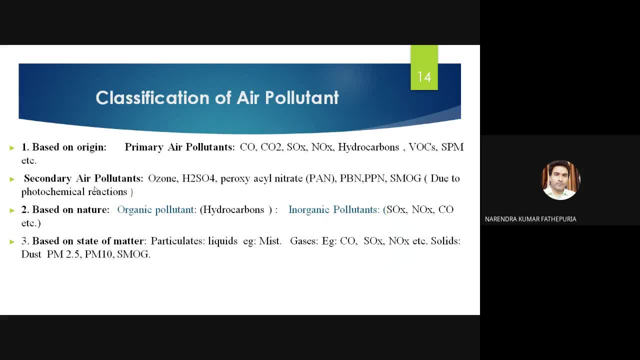 We have organic pollutants as well as inorganic pollutants, So organic pollutants like various hydrocarbons, right, And organic pollutants like SOx, NOx, carbon monoxide and various gases Based on the state of matter. also, air pollution has been decided divided. 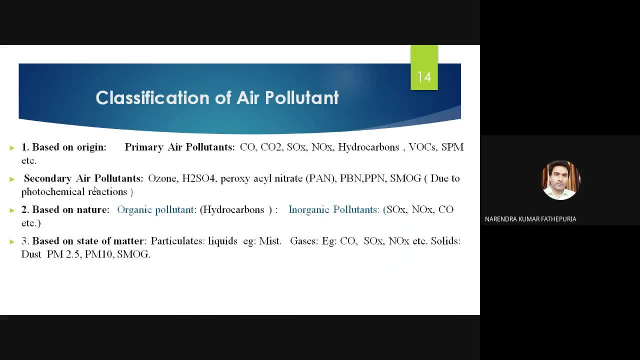 So there is a particulate which will be in the liquid forms. Some of the particulate matters will be in a gaseous form. Some of the particulate matters will be in solid form In that way also liquid, solid and gaseous forms also. we have divided based on the state. 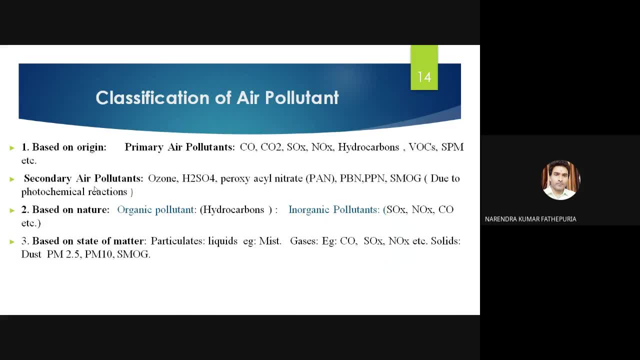 of matter. So the particulate which are in liquid forms, called as MISC, gaseous forms like carbon monoxide, SOx and NOx, And so, Okay, Solid pollutant. These are the various criterias of air pollutants. 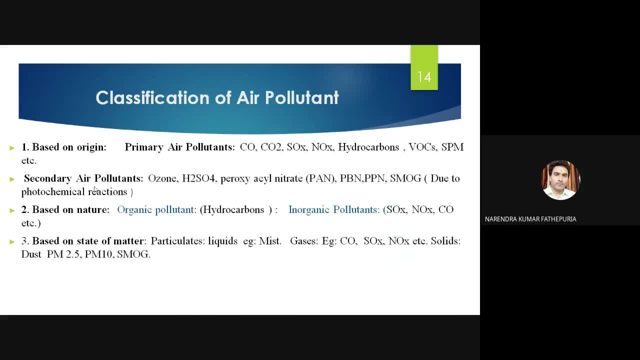 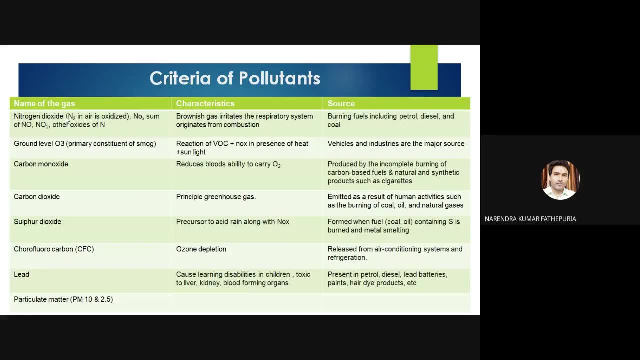 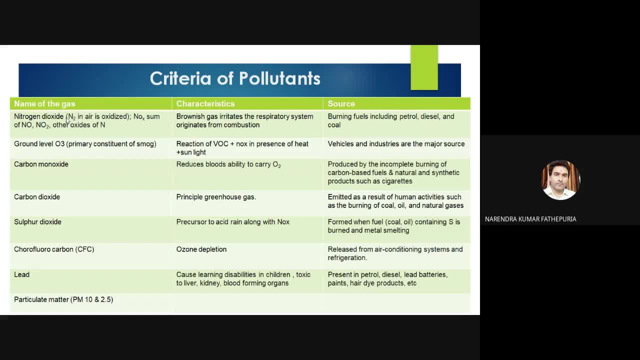 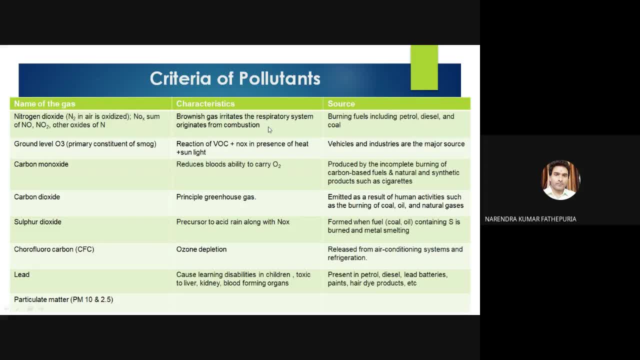 The color is brown for it. Gas irritate the respiratory system Or진ate from the combustion Sources, including petrol, diesel and coal. Ground level ozone, primary constitute of the smoke Reaction of VOC which is released from the combustion of the IC engines. 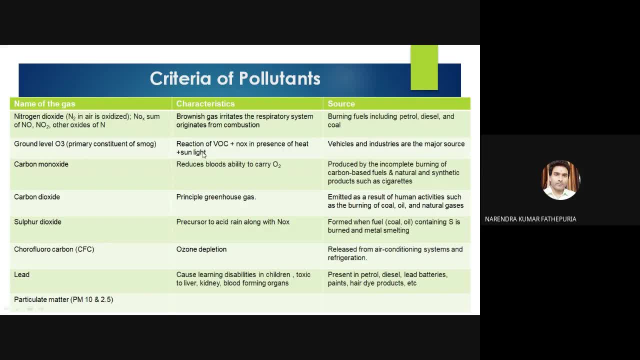 plus NOx. in the presence of heat and sunlight it will react it. it will form the VOC. Vehicular emissions and industries are the major source for it- Carbon monoxide. the characteristics for this carbon monoxide is very dangerous. it will like. 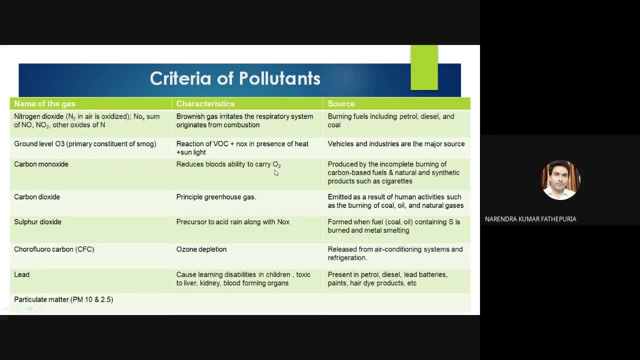 block your respiratory tract system, and then it reduces the blood ability to carry the oxygen. also, It is again produced from the incomplete burning of carbon, positively based emissions and natural and synthetic products such as cigarettes. and all that. One cigarette is having more than 4000 chemicals. 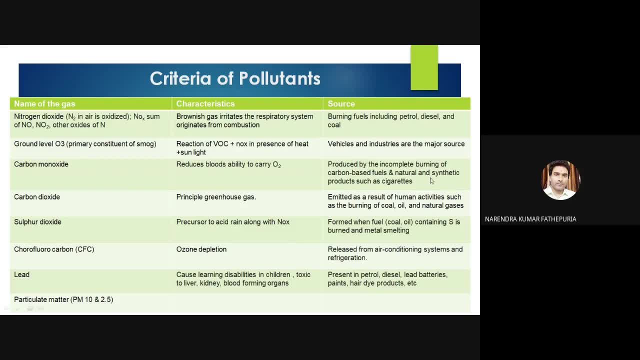 which are very harmful. There's a passive smoker as well as the active smoker, So it creates a lot of indoor air pollution. I will talk about the impact of the pollutions. Carbon dioxide, principal greenhouse gases, are the major constituent, major characteristic for it. 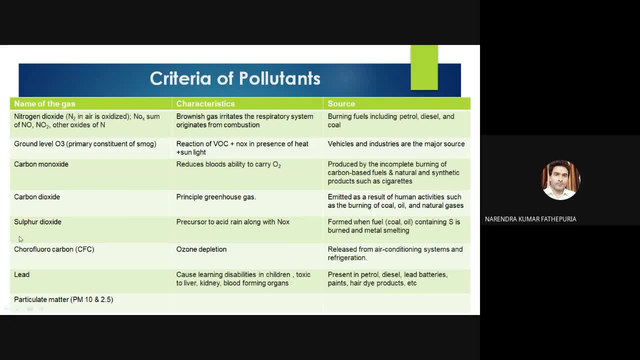 Emitted as a result of human activities such as the burning of coal, oil and natural gases. Sulfur dioxide because of to the acid rain. along with the NOx, sulfur dioxide is the main reason for the acid rain. Acid rain create a lot of water pollution right. 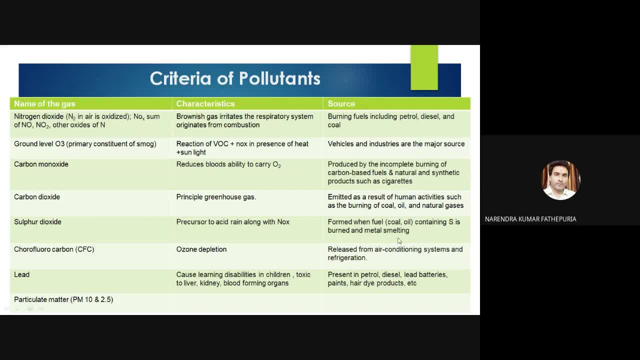 Pump when fuel- coal oil containing sulfur is burned and the metal is melting right. Then there's the chlorofluorocarbons, CFCs, which will be. the ozone layer is depleting because of the CFCs only. 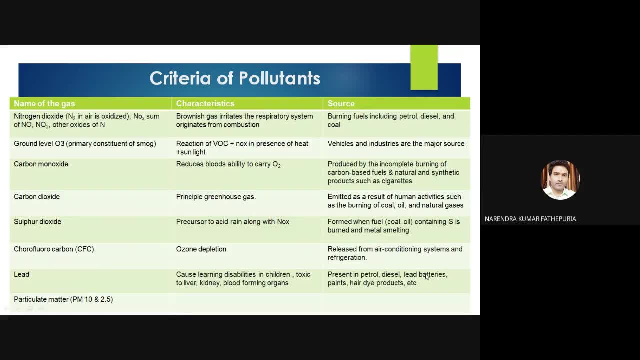 In greenhouse gases. you have your chlorofluorocarbons Released from the air conditioning systems and their physicians, their physician systems. There's a lead causing learning disabilities in children, toxic to liver, kidney failure as well as blood forming organs. lead is also very harmful. 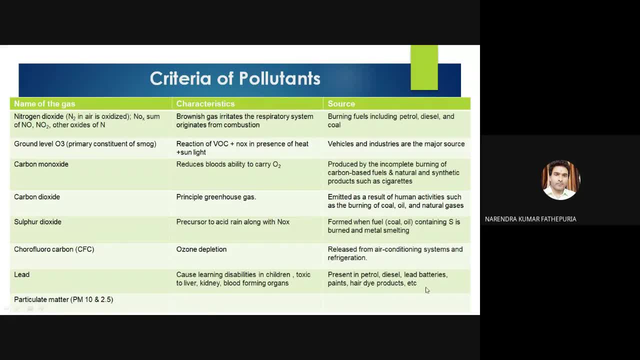 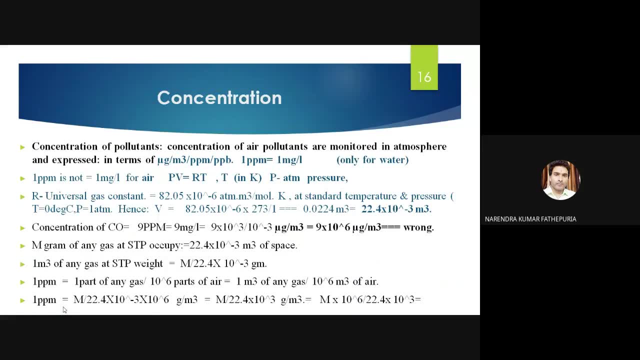 Resistant in petrol, diesel and lead, batteries, pens, hair dyes product and etc. There's a particulate matter- PM10, PM2.5, which is also released in continence: lead. okay, Before coming for this, I will just go for the impact. 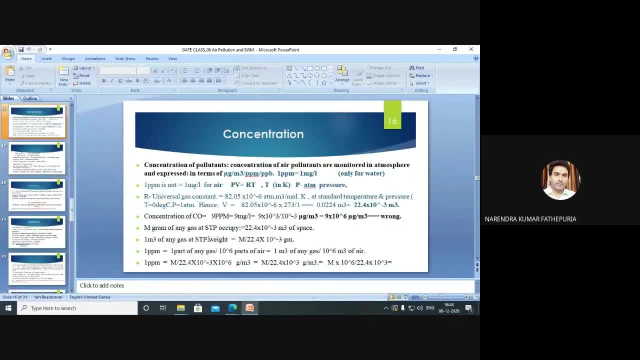 of air pollution. Then I will talk about all the numerical portions. what are the concentrations and all that. Just briefly, I will tell you this thing, Then I will, I will explain the impact of air pollution on planet and all that thing. 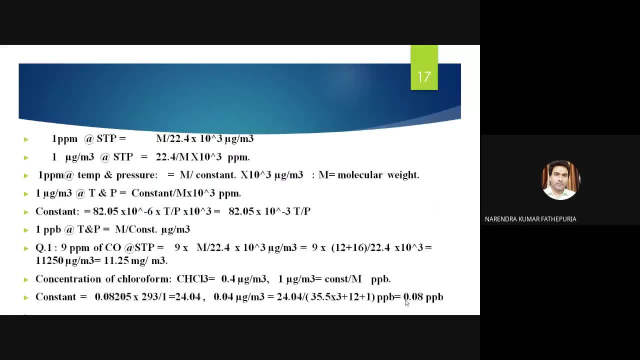 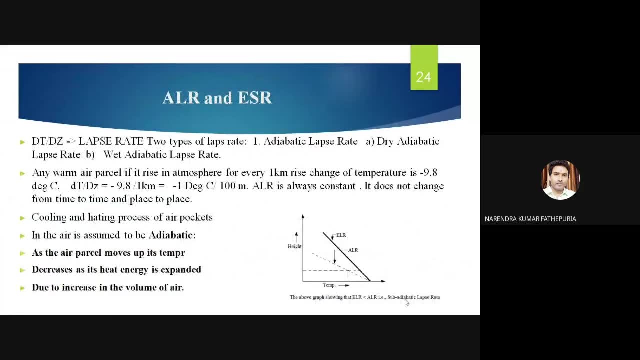 Then I will come for the numerical portion for this. These are the concentration formulas and all that, And these are the hydrocarbon dispersion and dilution techniques, The adiabatic lapse rate as well as the environmental lapse rate, we'll talk about it. 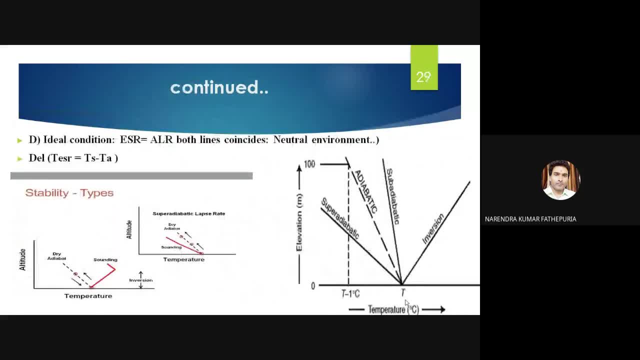 Stability of the environment. I will talk about it. And then there's the various dispersing mechanisms, how the pollutant is dispersed, how the pollutant matters. say, pollutants will particulate matters will disperse into the atmosphere. how to decide the stability? 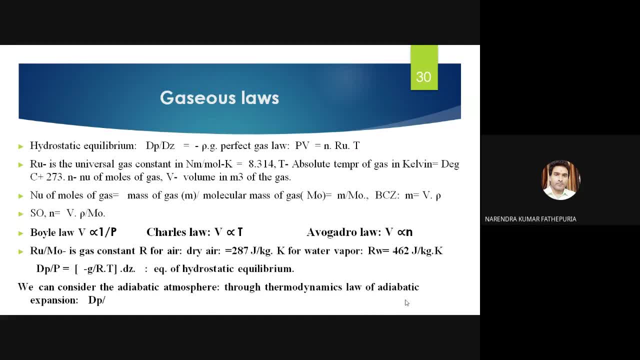 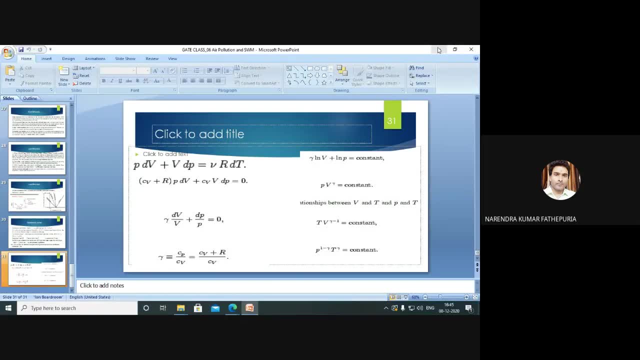 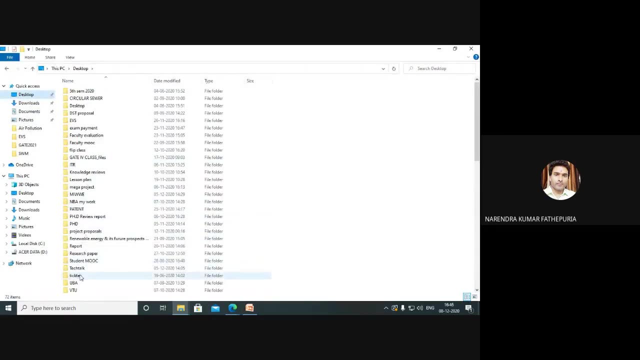 of the environment. right, And dispersion and dilution. how does it occur? right, The various gases law. I will talk, So I will come later for it. I will just go for the environment and pollution. So we are talking about the air pollution here. 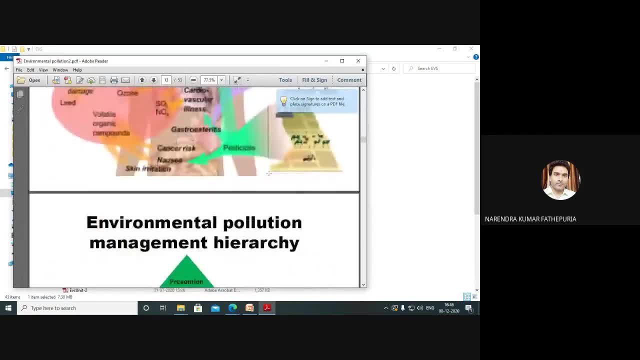 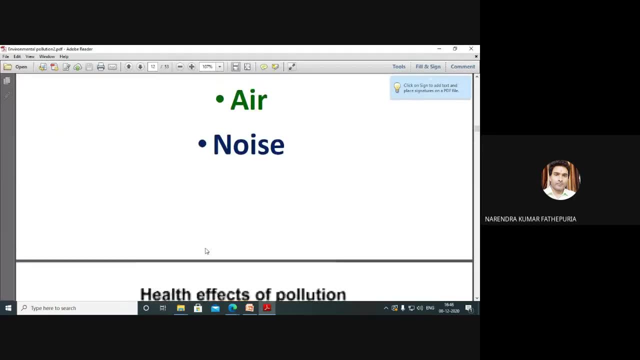 Yeah, These are the air pollutions, the health effect of pollution because of the air. actually, If we see here, air pollution in the air is really similar to air pollution in the real world. This is what we have. This is what I have seen. 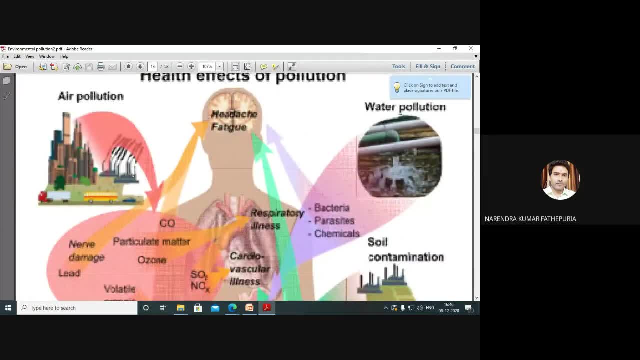 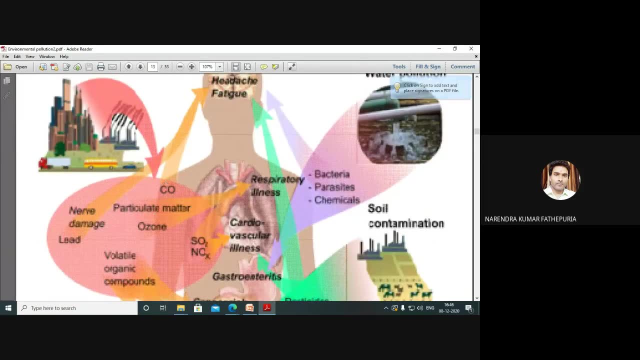 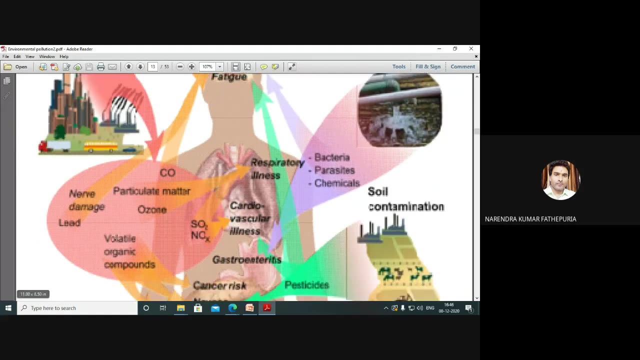 pollution which is released from various industries: automobiles, vehicles, even the commercial and construction activities, building, infrastructure development, various particulate matter, carbon monoxide, ozone, SOX and NOX, lead- It damages your nervous system. These volatile organic 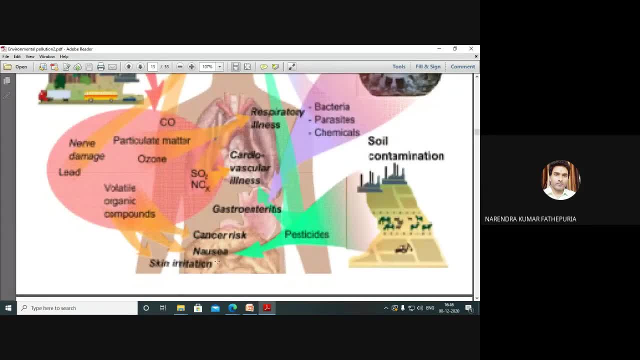 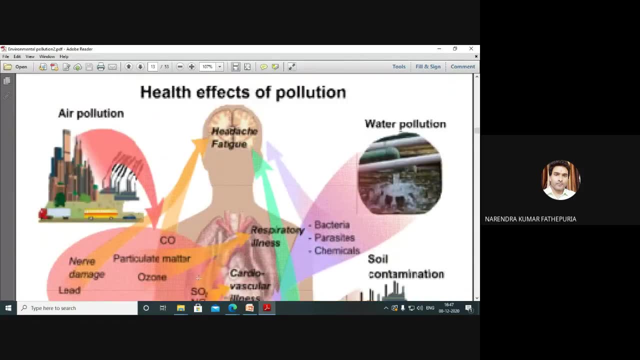 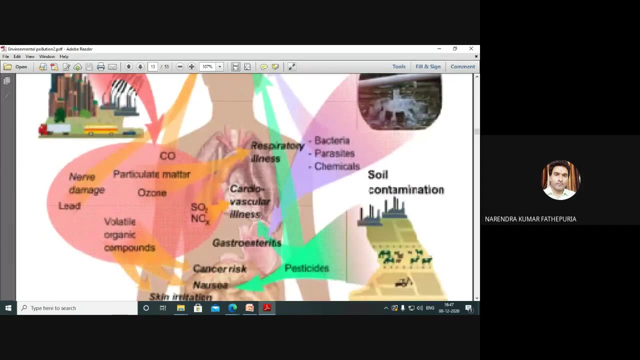 compounds, which also causes the cancer risk. skin irritations, various allergenic symptoms will come because of the VOCs. SOX and NOX causes various respiratory illness. your cardiovascular system also, the panel cardiovascular diseases also, because it will block your blood circulation systems and all that. There is various gastrointestinal diseases also, which 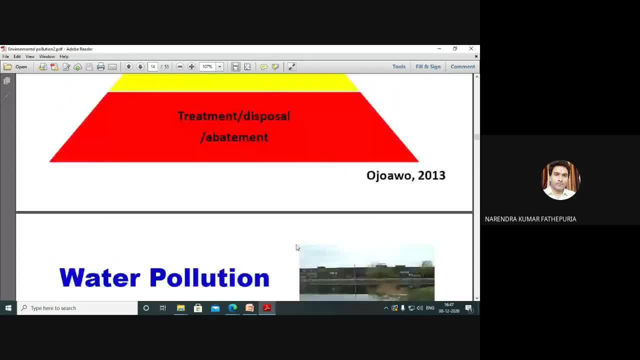 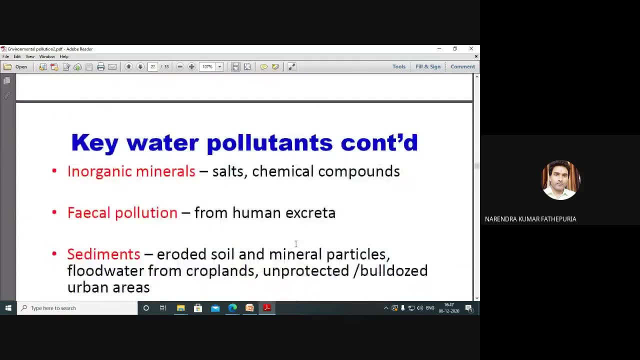 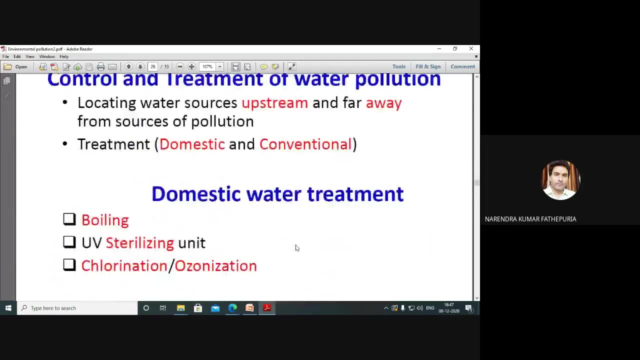 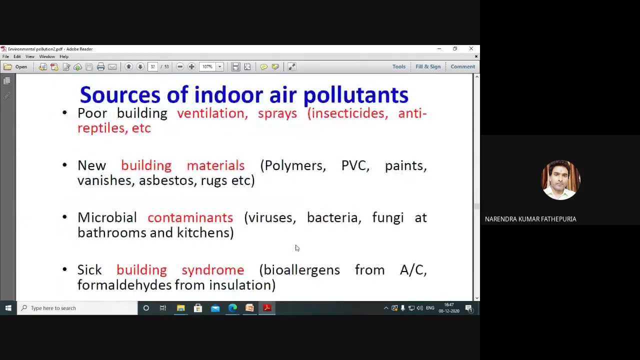 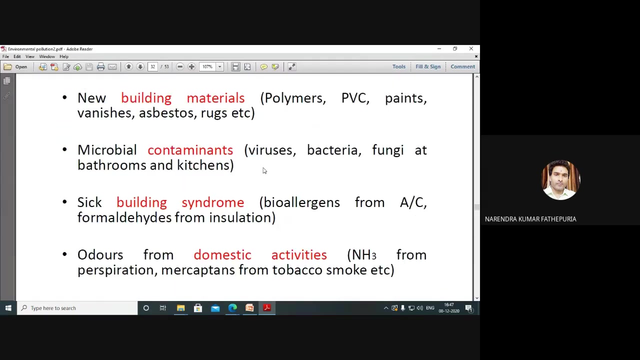 will come through the air pollution. I will come here about the air pollution part, So these we have discussed already. Now there are the sources. we have classified air pollution in two parts: indoor air pollution as well as outdoor air pollution. So the 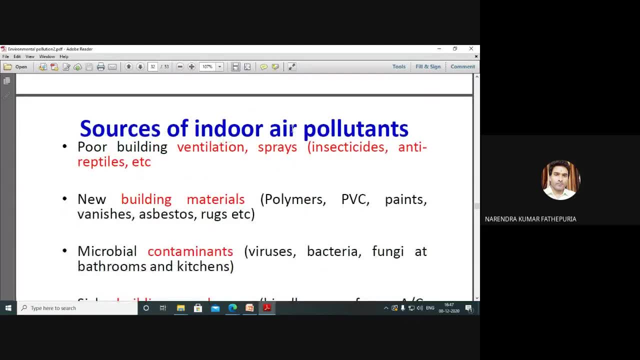 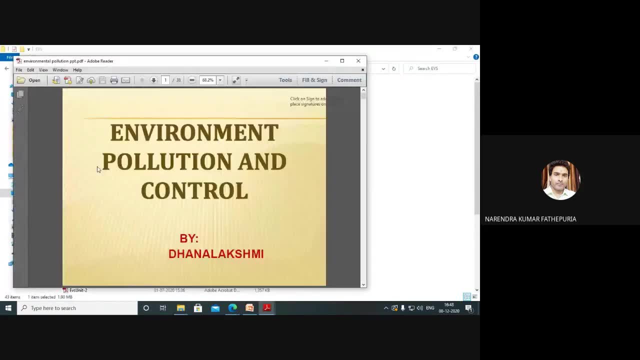 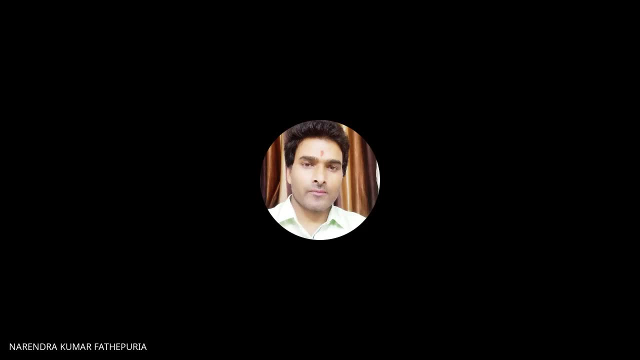 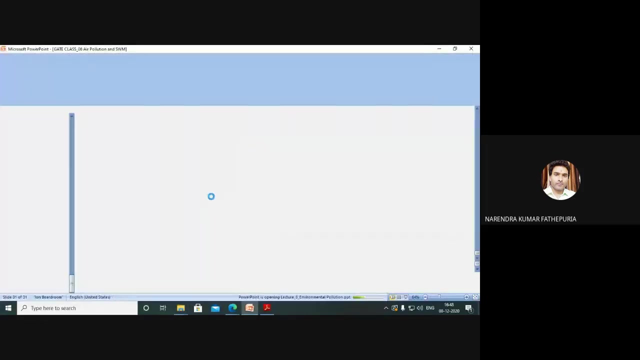 effect of air pollution. we will study First. we will see the sources of indoor air pollution or in your indoor air pollution part. Thank you very much for your attention. Thank you everyone. Thank you very much. Yeah, So you talk about here the factors which are usually associated with the air pollution. 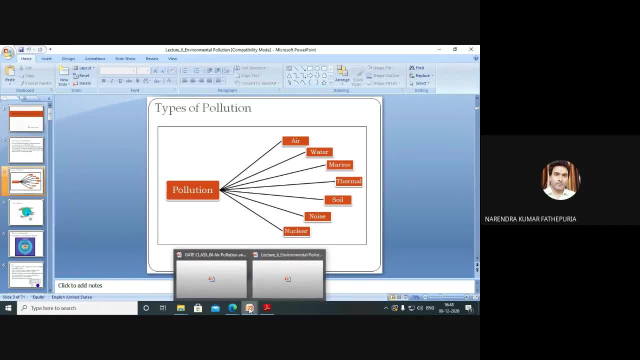 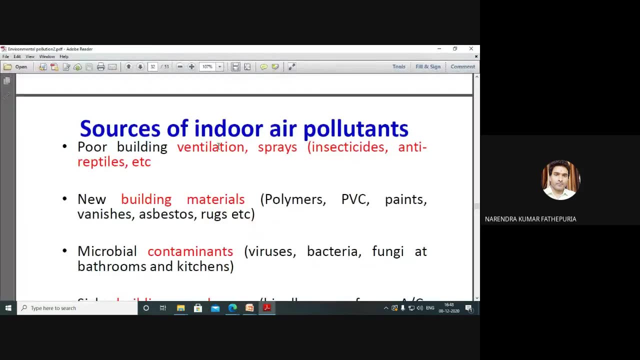 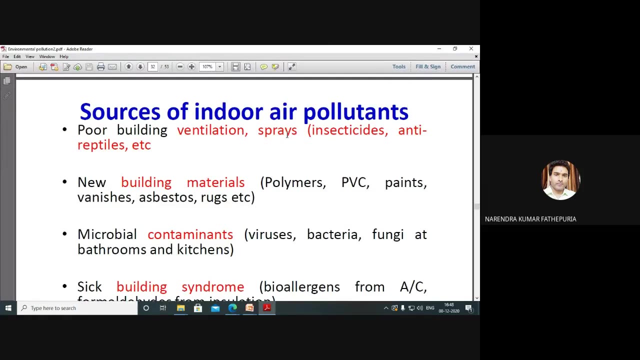 So talking about the sources, I mean the impact of your pollution. I will talk later. So these are the sources of indoor air pollution. There are two types of pollution as we have classified: indoor and outdoor. Because of the poor building ventilation with spray insecticide that you are using it for killing the insecticide in your house. 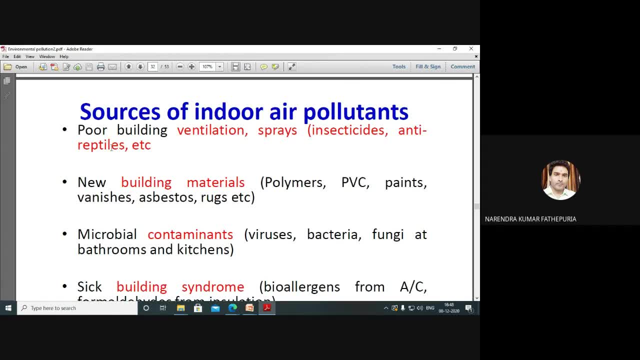 anti-reptiles that you are using at your home. it is having various chemicals, various chemical gases, New building materials that you are using in your constructing your house- polymers, PVC, pans, varnishes, asbestos- also causing indoor air pollution. 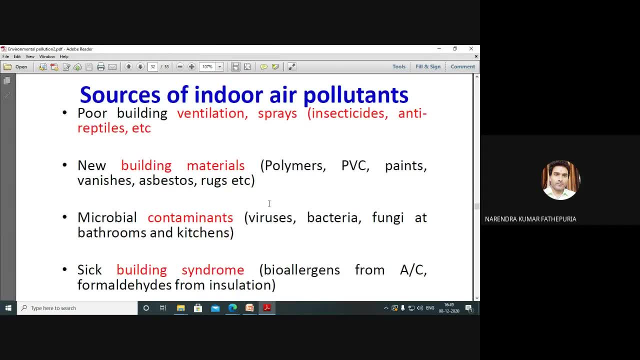 So what is happening? like the paint, whatever you are selecting for it, whatever the construction material you are using for constructing your house, it should be maintained. It should be maintained as a sustainable material and graded as a green building material So it can reduce the impact of the air pollution. indoor air pollution. 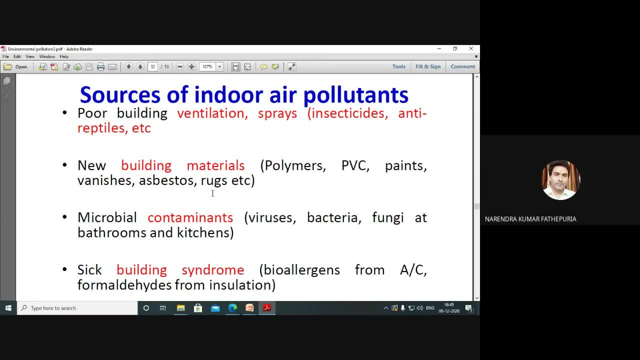 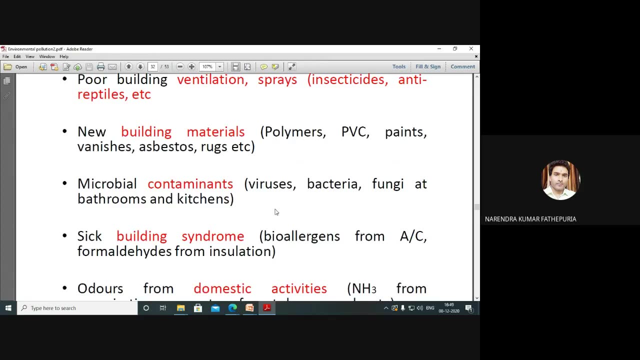 Because the color coding is very important. various colors will absorb the UV radiation more and the temperature also- Indoor temperature will rise, So it is very important while you are selecting your building material. Micro-bills contaminate various viruses, bacteria, fungicide. 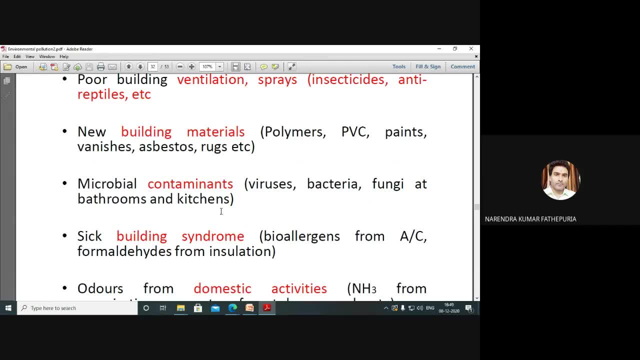 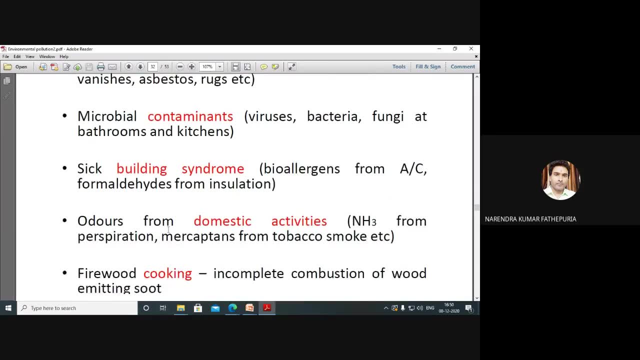 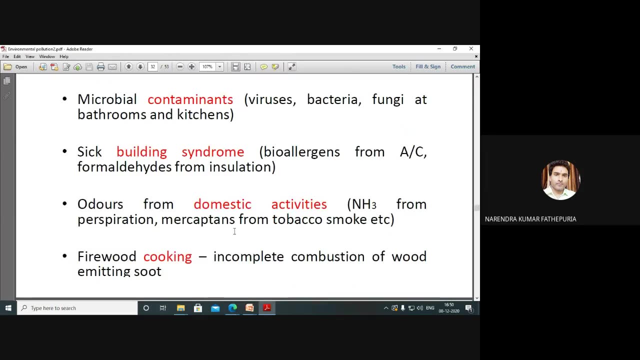 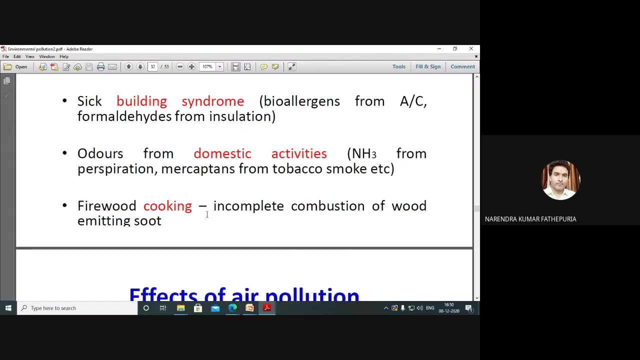 So it is very important while you are selecting your building material. So it is very important while you are selecting your building material, It is very important while you are selecting your building material. iphíd pregunté 0 0b A. How do you select your building material? 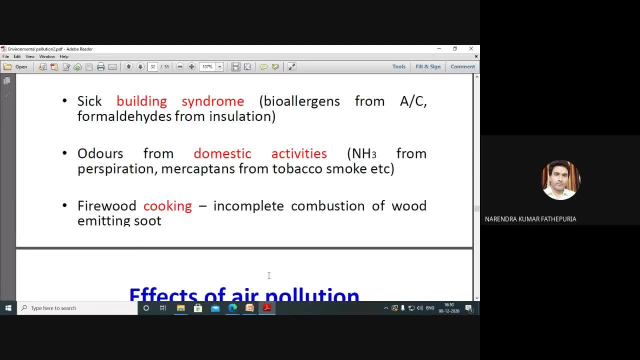 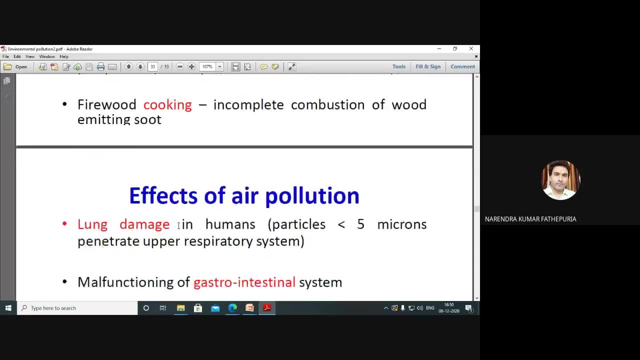 Incomplete combustion of wood, emitting force, causing soot, which is having carbon monoxide and carbon dioxide, which will reduce the atmosphere In your old days, in villages, and all that, firewood cooking is common, which causes a lot of air pollution, And these are your effects of air pollution. 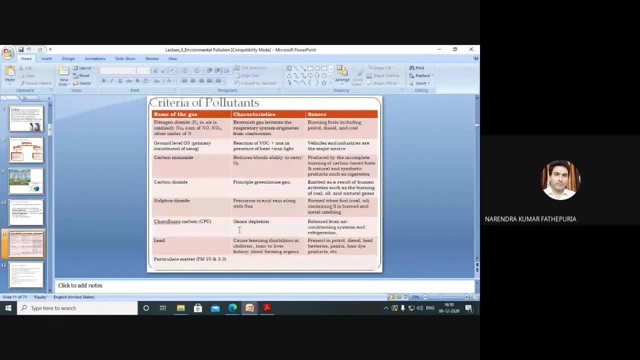 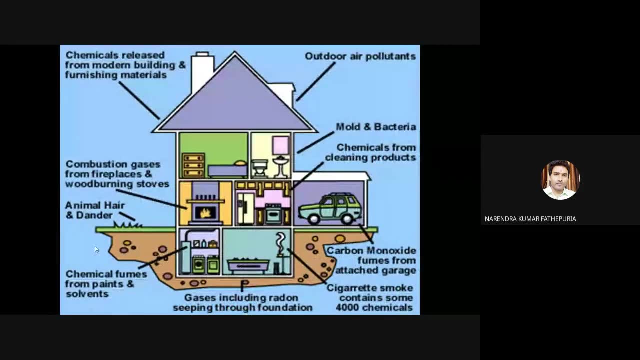 So one house itself. you see that how much emissions of we are releasing it. and for the indoor air pollution, The chemical released from modern buildings and furnaces, buildings causing air pollution, indoor air pollution. Then combustion of gases from fireplaces and wood burning stoves in your kitchen. 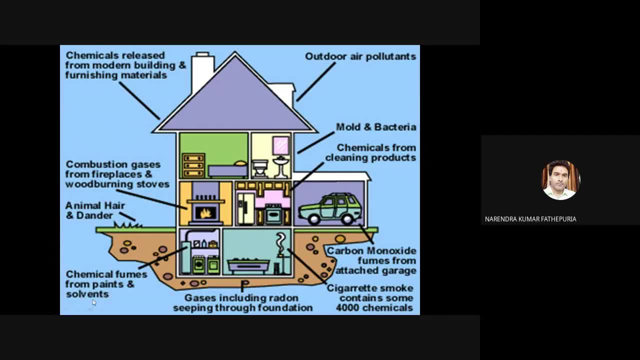 Animal hair in renders chemical fumes from pens and solvents releasing Gas is also released. Gas is including red on seeping through the foundation. Through the foundation the percolation and infiltration of gases is happening like seepage formation. Then various gases released from carbon monoxide fumes from attest garbets garras. 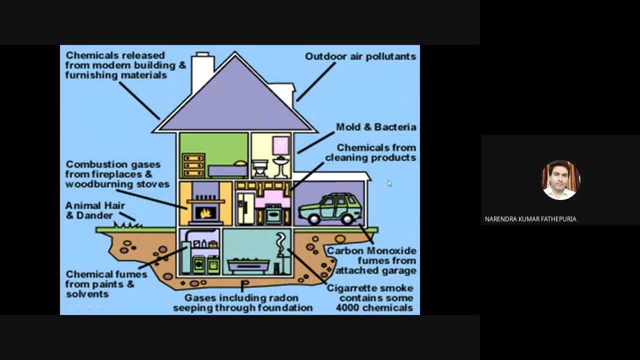 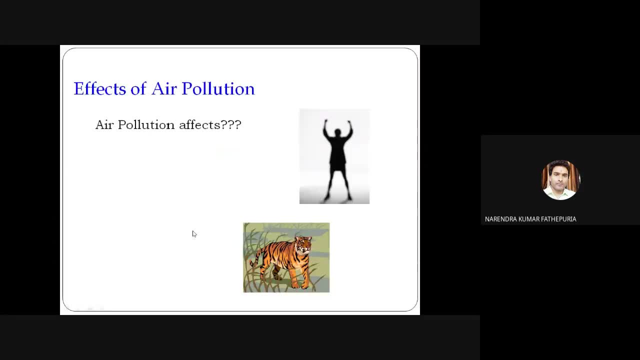 Cigarette smokes contain more than 4000 chemicals, The chemicals from your cleaning products, mold and bacteria, outdoor air pollutants. These are the responsible things. So effect of air pollutions are there on human health, Animals as well as plants, as well as the material as well as the environment. 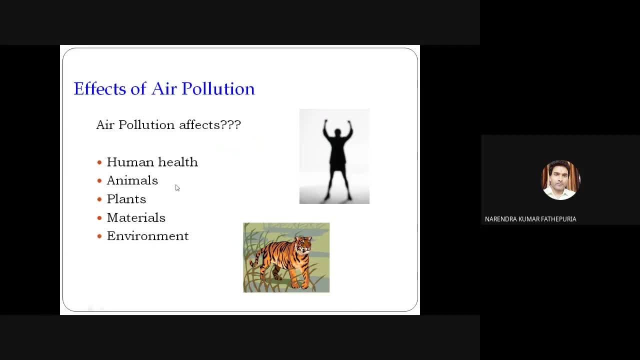 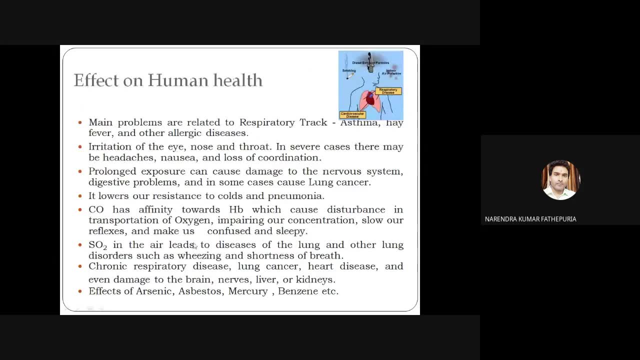 These are the severe effects of air pollution on human health in animals, plants, material as well as the environment. So I will go in for one by one about the human health. first Effect on human health. The main problems are related to the respiratory tract. 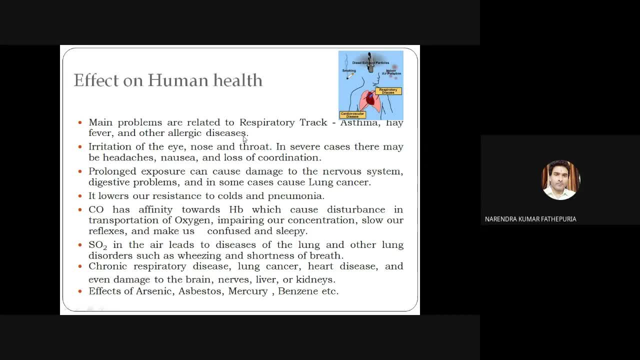 Asthma, hay fever and other allergic diseases. Irradiation of the eyes, nose, throat. In severe cases there may be headache, nausea and loss of coordination. Prolonged exposure can cause damage to the nervous system, Digestive problems and, in some cases, causes lung cancer. 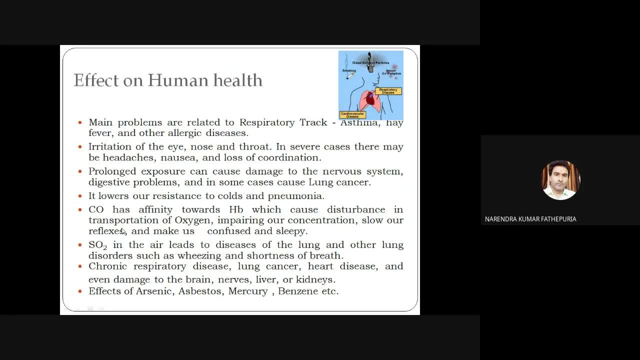 It lowers our resistance to cold and pneumonia. Carbon monoxide has affinity toward HP, which causes disturbances in your transportation of oxygen, Impairing our concentration. It also relaxes reflexes and makes us confused and sleepy, So carbon monoxide is very harmful. 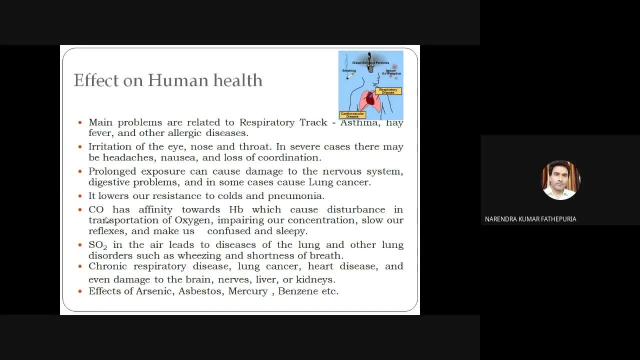 It causes cardiovascular diseases. also, Sulfur dioxide in the air leads to disease of the lungs and other lung disorders such as wheezing and shortening of breath, Chronic respiratory diseases, lung cancer, heart diseases, Even damage to the brain, nervous system, liver and kidney. 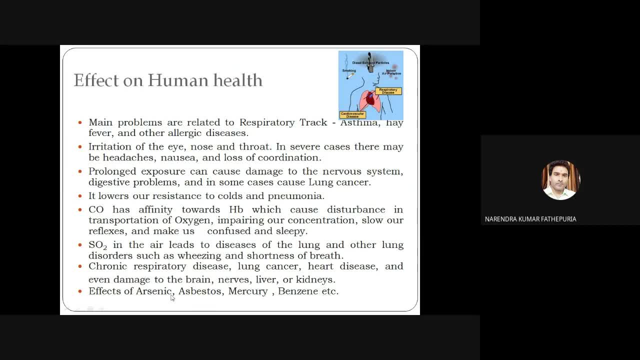 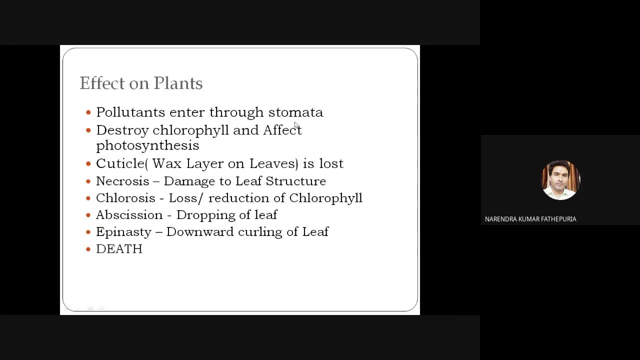 Effect of arsenic, asbestos, mercury and benzene. These are the toxic substances, which poisonous substances, which causes lot of problems for the human health. Then there are the effects on plants also. Pollutants enter through stomata. These air pollutants enter through the stomata and leaf. it is there. 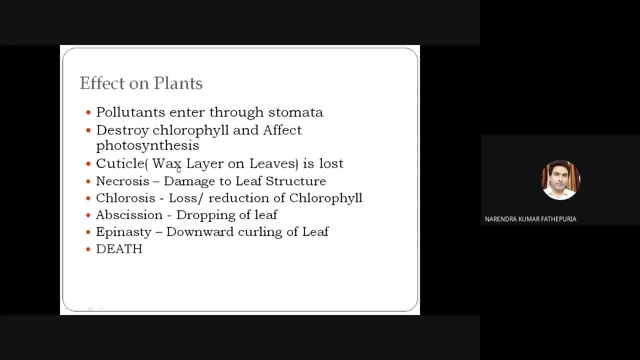 Destroy the chlorophyll and affect the photosynthesis process. Photosynthesis process is the only process. Through this you are getting a fresh oxygen into the atmosphere through our produces, Like plants In the making process of this photosynthesis process, the food making process of plants. 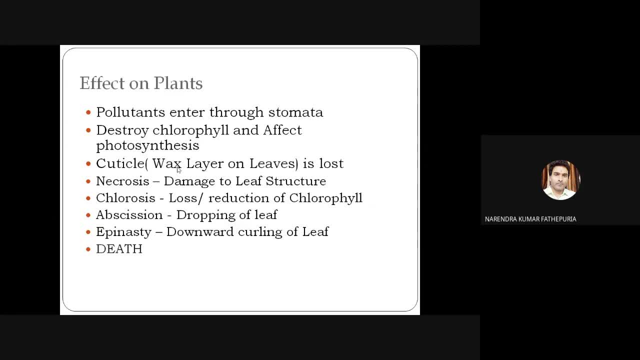 What they are using it: The huge amount of carbon dioxide, sunlight, various nutrients. they are absorbing from the soil And the water that is needed. So they are. They are using it to make a fertilizer for trees and for plants. So to make a fertilizer it is very important to have. 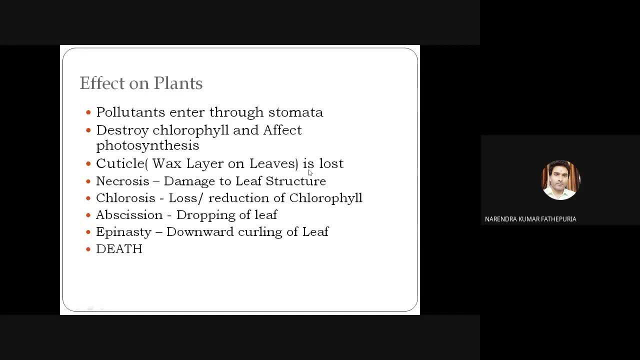 What they are using it for. So this is the cleaning process of plants. So we are using it for a fertilizer for plants. So we use it for a fertilizer, to make a fertilizer. So it is very important to have it here at home. 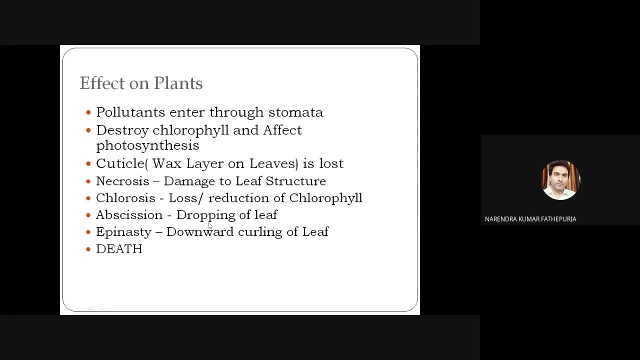 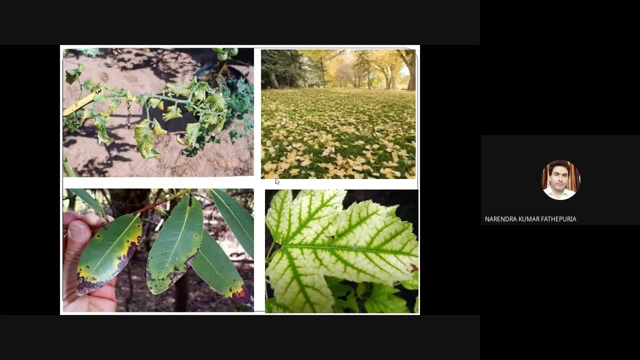 For the hike, for the cross-country, But it's also used for a little bit of food. This is the durch or the не durch For the superatox, for the depletion of the soil. These are the various diseases which is happening because of. 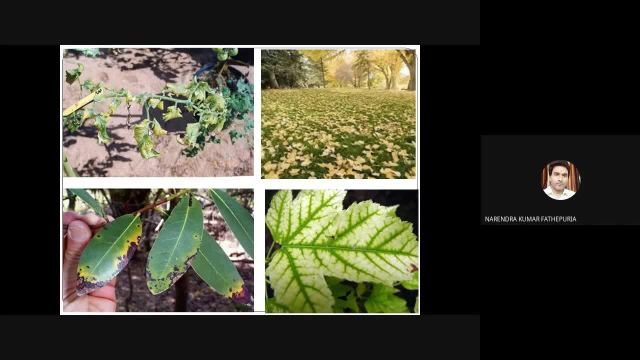 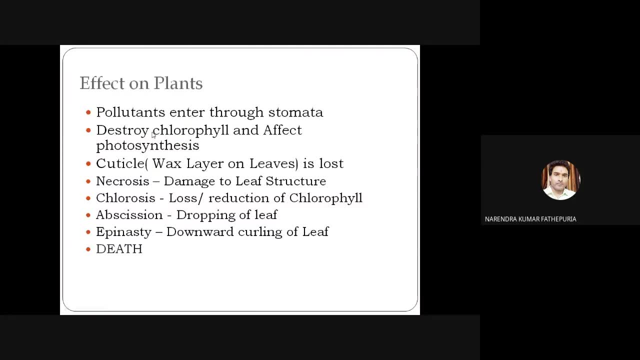 the air pollution, The color degradation is happening, the leaf is dying, right, You see that for various plants, right? So these are necrosis, chlorosis, abscission, these are leptin STDs. these are the various diseases, various. 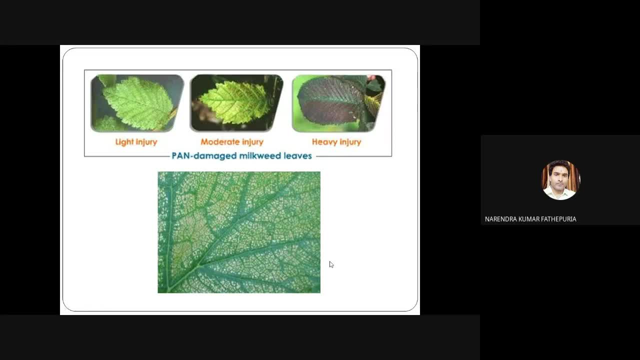 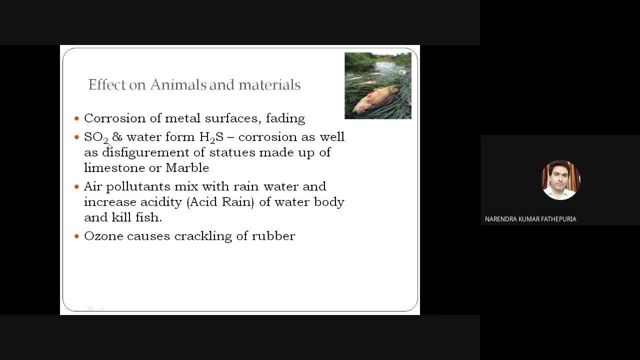 impact of air pollution. These are the injuries and because of the pen, pen is damaging the milkweed leaf. light injuries, moderate injuries and heavy injuries. okay, The effect of animals and materials are also severe: Corrosion of metal surfaces, fading the color of our buildings, right, Our 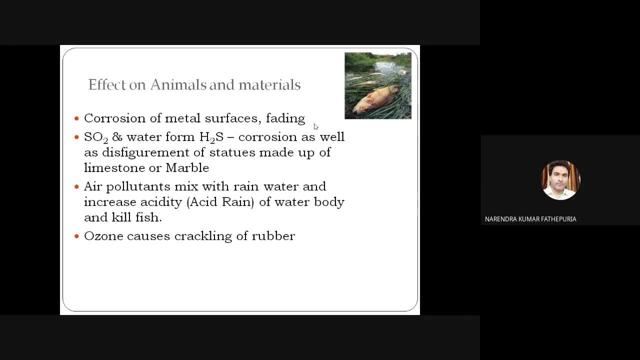 historical monument like marbles. degradation is happening because of the sulfur dioxide in H2S. Because what is the repeated abrasion and corrosive action? what is happening? The color is converting into the pale yellow color. right, The slow degradation is happening for. 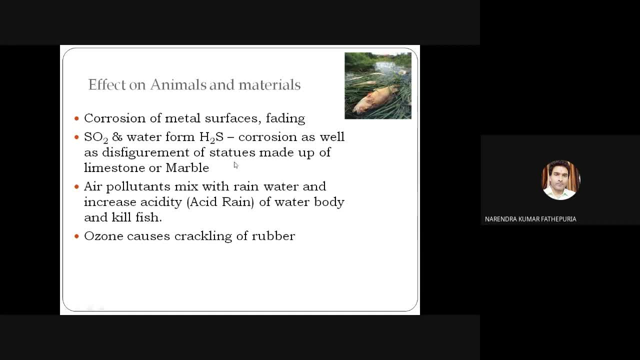 our historical monument. That is happening. The disfiguration of the statue is made up of limestone and marble. Air pollutants mixed with the rainwater increases acidity also. This is a main reason for the acid rain for water body and it causes the water pollution and 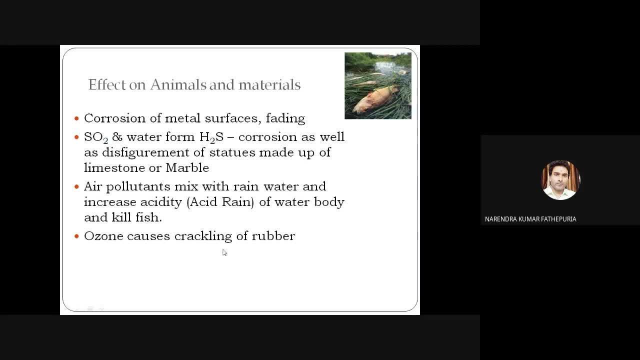 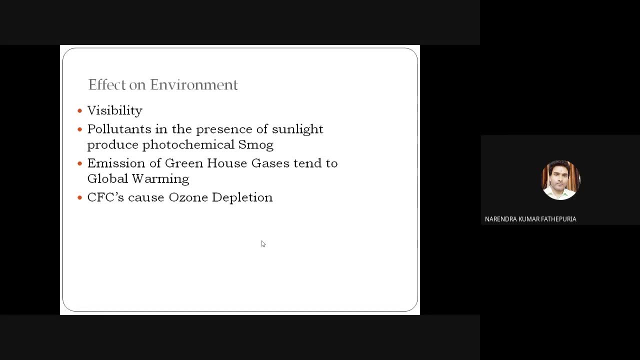 kills faces, water, all the water, animals, Ozone causes, cracking of the rivers, ozone layer depletion. UV radiation effects are quite common right And then effect of environment, like visibility. Global warming is also one of the big reasons for this, Because of the greenhouse gases, the 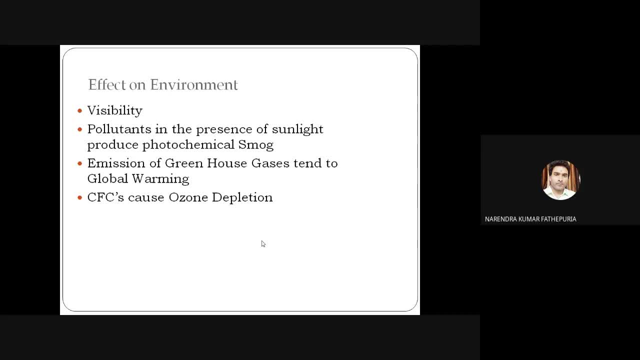 global temperatures. warming is happening right. Temperatures are rising rapidly. Our ice glaciers are melting right. Emission of greenhouse gases causing chance to the global warming. Chlorofluorocarbon causes ozone layer depletion. Polytens in the presence of the sunlight produces. 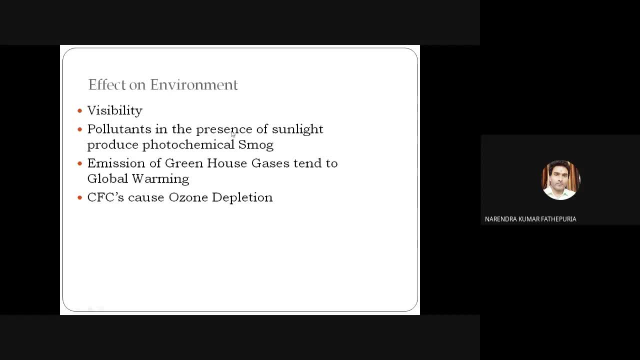 photochemical smoke. This photochemical smoke is very harmful In the presence of sunlight, produces photochemical smoke and that is visibility will be less and then, while you're breathing this toxic air, again a lot of problems will be happening. yeah, 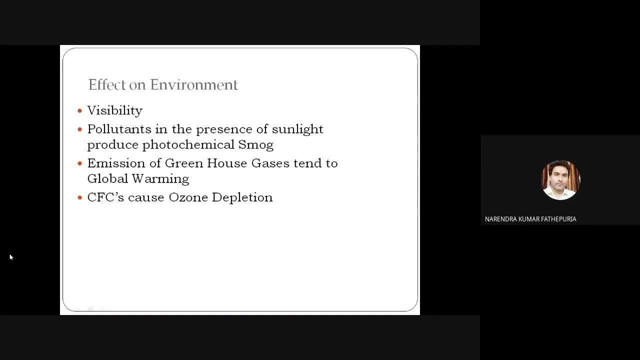 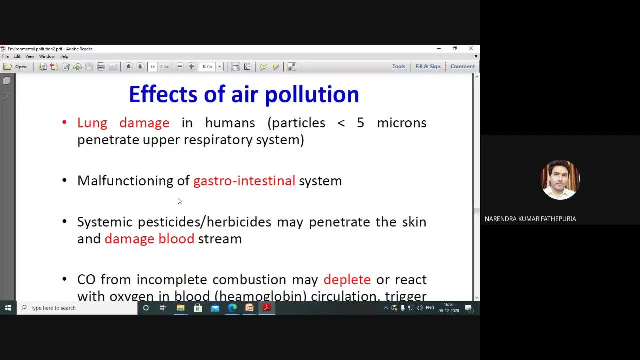 The National Ambient Air Quality Standard. I will talk later. while I'm going for the solution. First you have to understand the severity of the problem, The severity of the pollution. So this I already talked about it: Lungs damage, gastrointestinal systems or systematic pesticides, herbicides may penetrate in the 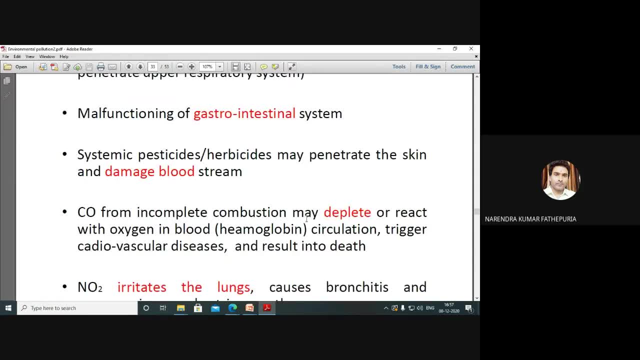 skin and damage blood cells. Carbon monoxide from the incomplete combustion may deplete or raise with oxygen and blood cells And hemoglobin circulation and trigger cardiovascular diseases. result into death. Nitrogen dioxide irritates the lungs, causing bronchitis, and pneumonia may cause trigger. 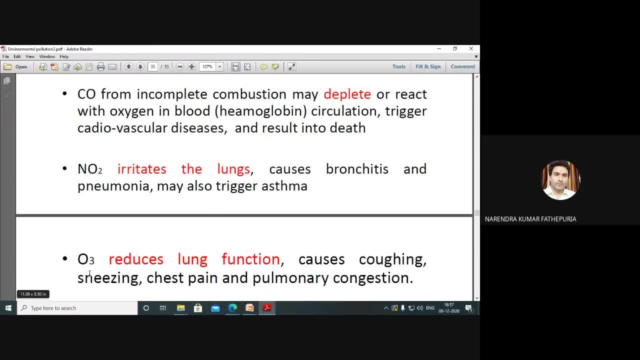 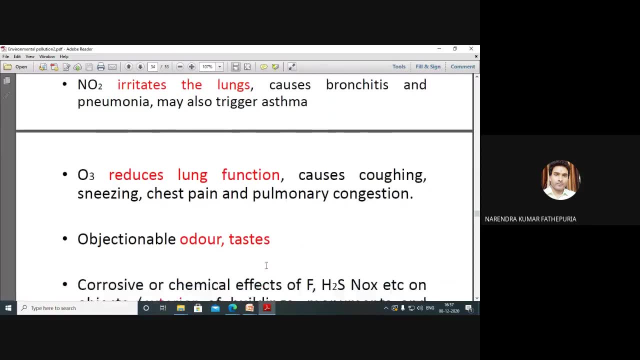 asthma right These? I have already spoke about it. This is: the ozone reduces the lung function, causes coughing, sneezing, chest pain and pulmonary congestion. Objectionary will order in taste, Corrosive or chemical effect of fluoride. 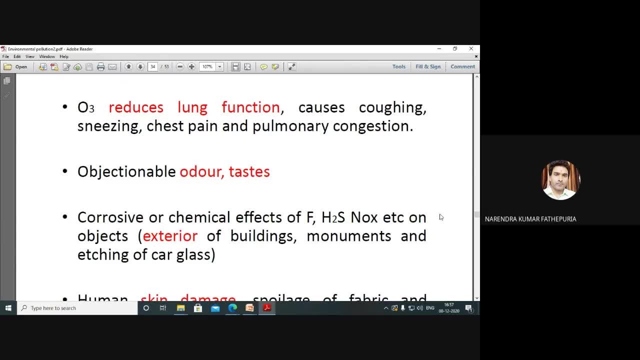 fluoride, as well as hydrogen disulfide or NOx, ETC on objects or any other toxic substances. This is the most common cause of the problem. The most common cause of the problem is the deterioration of the building and monuments right, Or deteriorating of these. 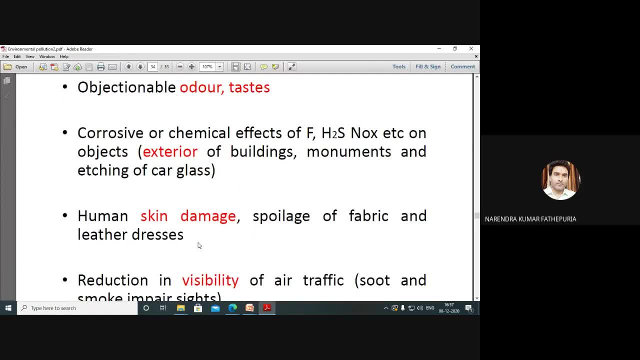 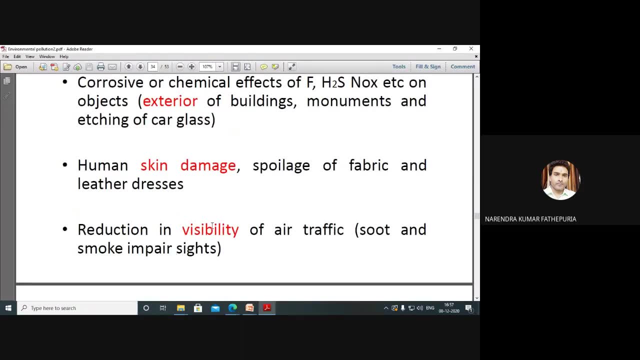 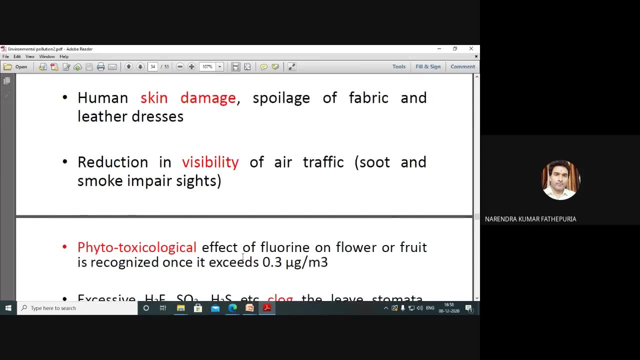 monuments, Human skin damages, spoilage of fabric and leather, various insecticides and various cosmetic products, causing the skin cancer problems. right, So there are the eight type of polygons which are responsible for skin cancer Reduction. visibility of the air, traffic, soot and smoke, impure. 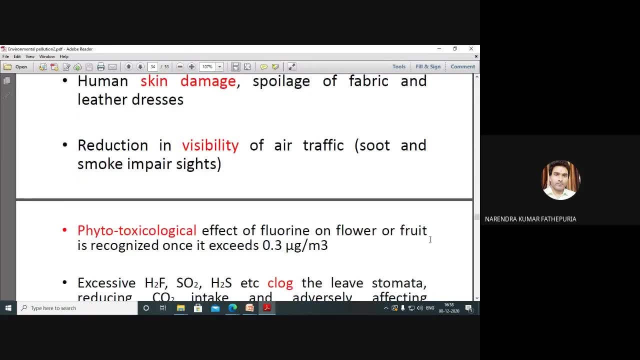 skin and mucus. The most common cause of the problem is the effect of fluoride on the flowers, as well as the fruits and plants. Once the fluorine contained exceeds 0.3 microgram per cubic meter, it creates a phytotoxicology effect which will 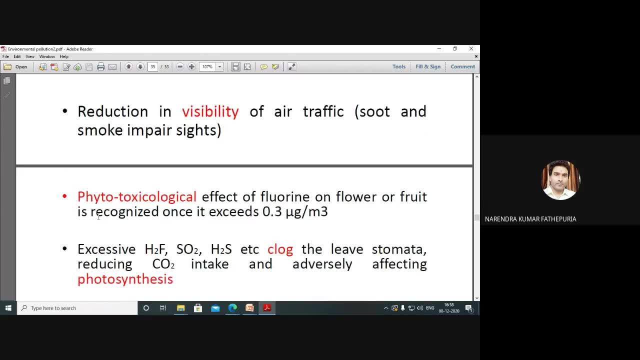 transmit from the various trophic labels, from primary consumer to secondary and tertiary consumer and then decomposes. So these pollutants will keep transmitting from one body to another body and it creates a problem. It creates a lot of problems for the flowers and fruits And then excess of hydrogen. 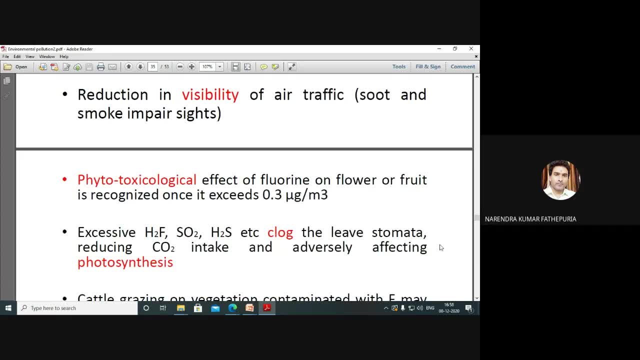 disulfide, sulfur dioxide, hydrogen disulfide- clog the leaves stomata, as I told you about the plant effects effect of pollution on plant producing carbon dioxide intake and adversely affecting the photosynthesis process, As I told you that this photosynthesis. 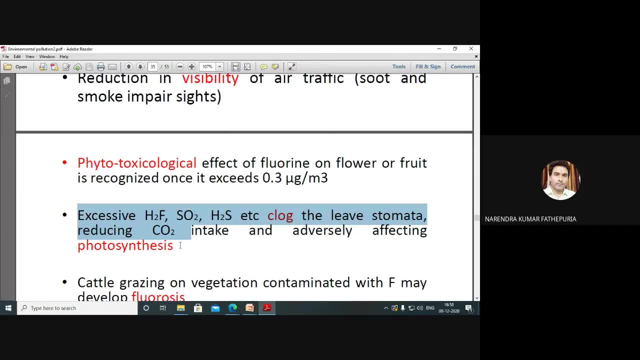 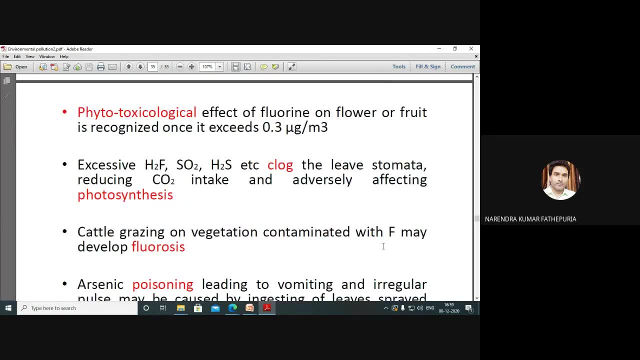 is the only source of oxygen. If the photosynthesis process is disturbed, you will not get the sufficient amount of oxygen from the plant. These are the produce. Cattle grazing on vegetation contaminated from fluorine, they develop fluorosis. This is the 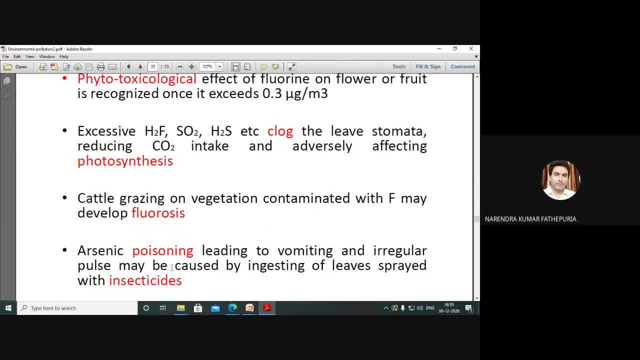 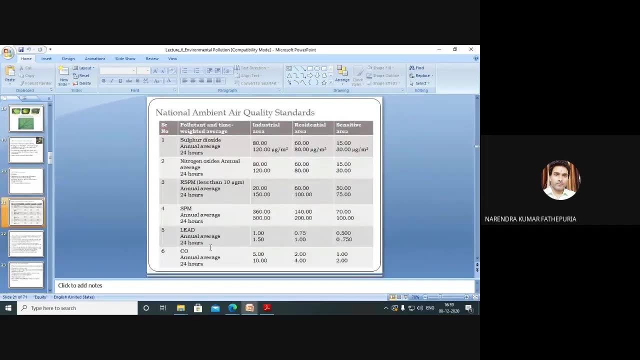 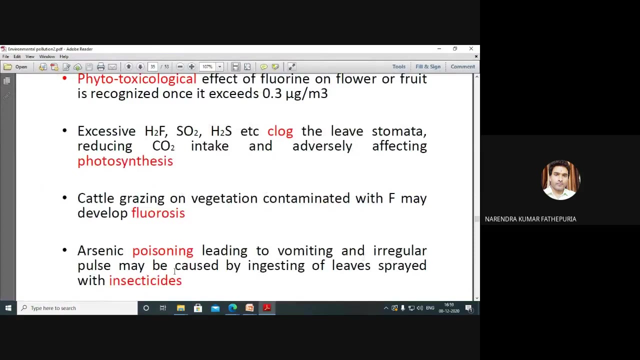 and then um, arsenic poisoning, arsenic, lead, um, as i told you about the lead contaminated particles, now these are the things like um, where it is. yeah, so these are, uh, the main pollutants. arsenic poisoning, leading to the vomiting in irregular pulse, may be caused by by ingesting of lead sprayed with the insecticide, causing a lot of. 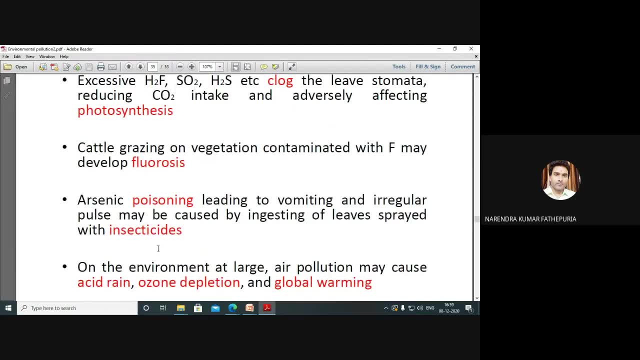 problems, and bioallergenic also is a problem on the human being. 80 population is suffering for the allergenic symptoms. allergy may be in the form of this skin allergy, breathing allergy, and all that on the environment. at large scale air pollution may cause the acid rain ozone layer depletion. 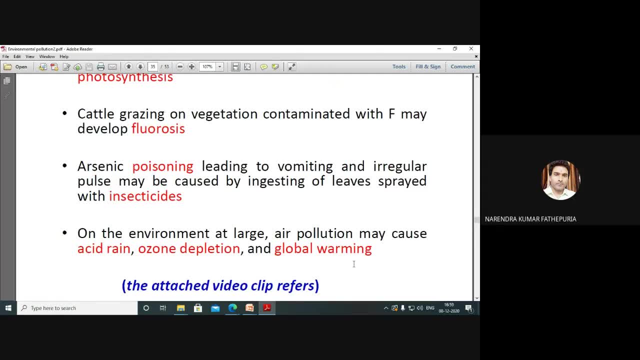 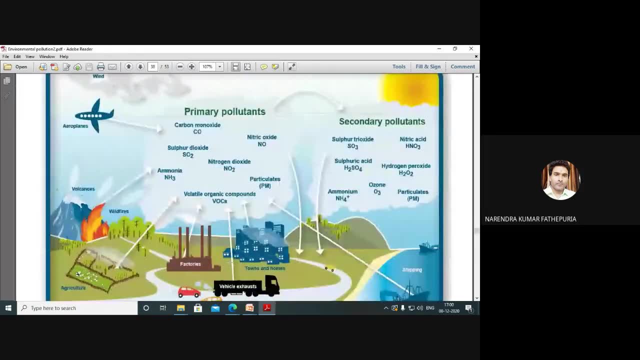 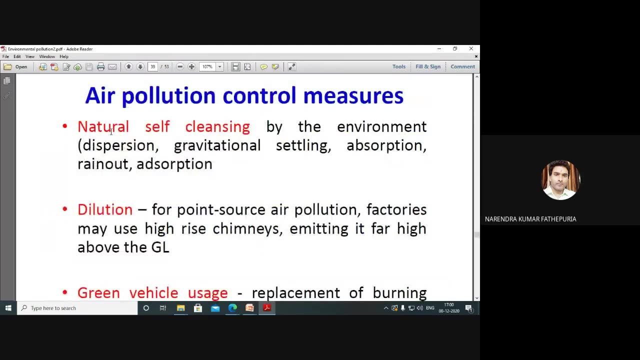 global warming. these are the well-known um worst environmental impact- uh acid rain and ozone layer depletion and global warming causing because of the air pollution of lead pollutant. i have already discussed about the polar primary pollutant as well as the pollutants. now i will come about the air pollution and control in measure. 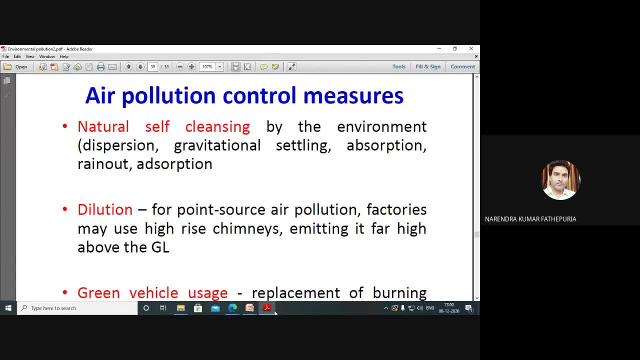 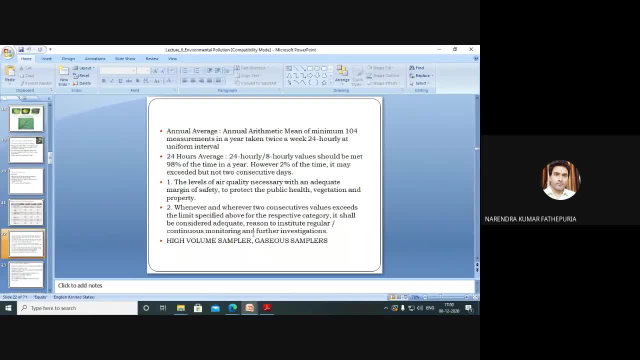 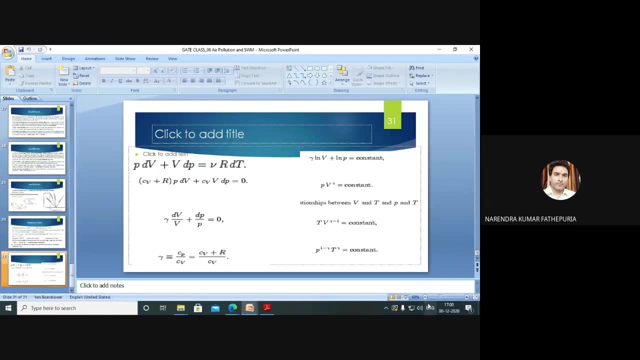 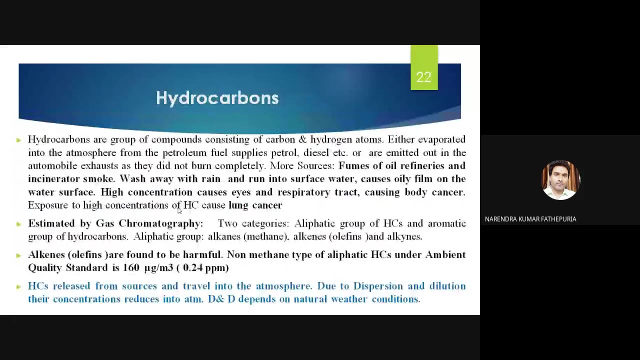 so measurement is important. okay, once i go for the measurement part then i will come for this uh control measurement part of pollution. okay, yeah, so first is, as i told you, the concentration play a very important role. you, while you're annually measuring the fruition, you have to understand about the concentration, concentration generally. 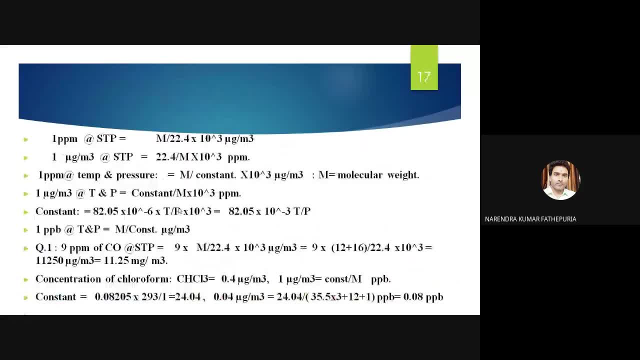 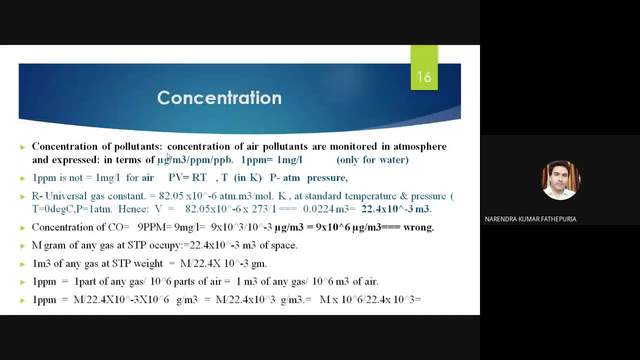 like what is like several nell. yes for this really simple rule for the concentration you have to see about the laser in less amount, like if you see, generally in mc per liter. we talk in water, no milligram per liter, right in water. in terms of gases, there's a. this is different, right, in terms of gases, pollutant, you are basing. 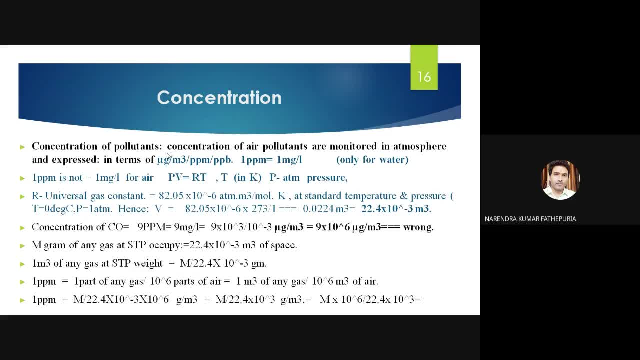 it. the concentration of pollutants. the unit will be also different. here. the concentration of air pollutants are monitored in atmosphere and excess in terms of microgram per cubic meter. yeah, ppm or ppv sometimes, the microgram per cubic meter is most common unit. while you are going for particulate matter, concentration, sox, concentration, anox, concentration, everything you 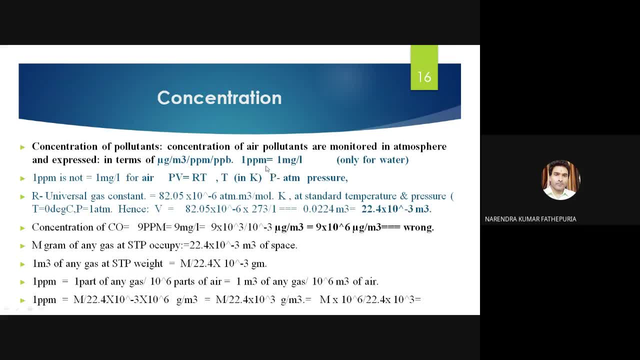 are going to measure in microgram gram per cubic meter. so generally one ppm is equal to one mc per liter. right, only for the water. but one ppm is not equal to one mc per liter in terms of air or gases. so we have a gases law that is: pv is equal to rtp, is the temperature in kelvin which. 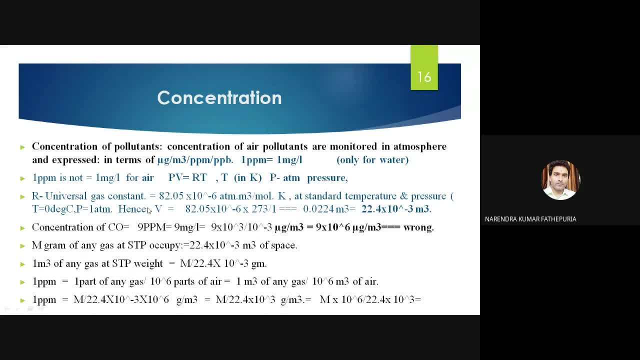 is the atmospheric temperature, is the uniform universal gas constant, which will be 82.05. there are the four laws for gases i will discuss later. 82.05 times or minus six um uh, atmosphere. uh into cubic meters by mole, into kelvin, right, so so this is um the whole unit for it, uh, for the. 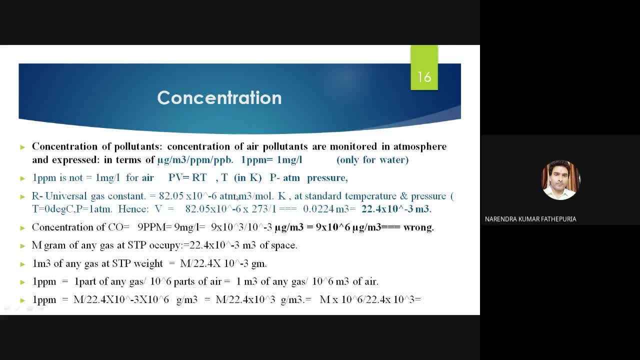 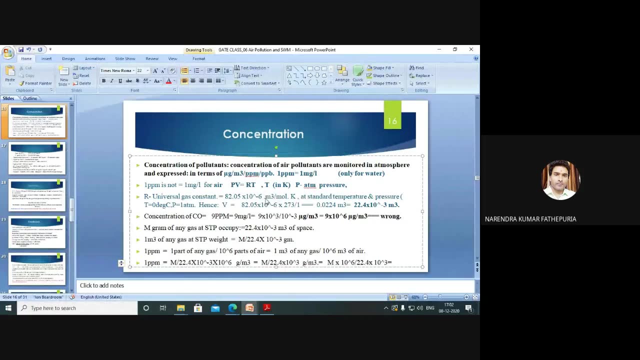 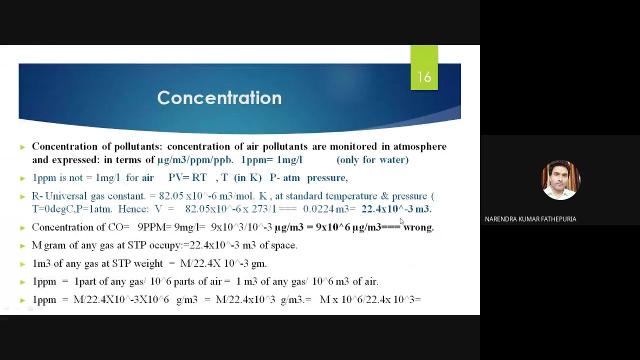 gas constant at a standard temperature and pressure. yeah, now it is fine, this is the unit for the gas constant. and then at standard temperature and pressure. stp, stv. i will call stp from now on. what is the standard temperature and pressure? that is standard atmospheric and room temperature. 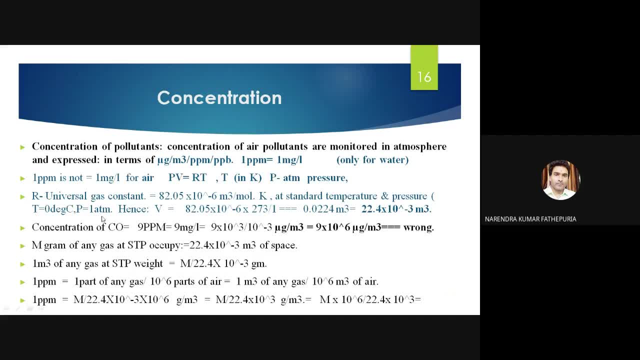 in atmospheric pressure. p, we are taking a degree celsius. p is one atmospheric temperature, we are taking it, and v is the volume. uh, you can get the gasses volume by using this formula: v will be equal to divided by one one. p will be in the right hand side and r is given 82.05 into 2 sixty. 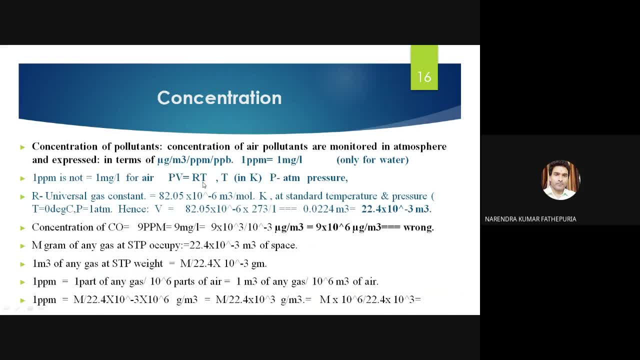 multiplied with t, multiplied with the z and two, seven to three, diesel room temperature right, and then divided by one, you will get it as twenty two point four into ten to the minus t suchen. this is a twenty two point four into ten to the minus you that values. for respective tables of the으�, הר, fr, Horse temperature and volume. one, t will be in the right hand side and r is given eighty two point zero 5 into t minus 36. multiplied with t, multiply with 273, it's a room temperature right, and then divided by one, you will get it as a twenty two point four into ten to the minus six m Ahp. this is a twenty two. 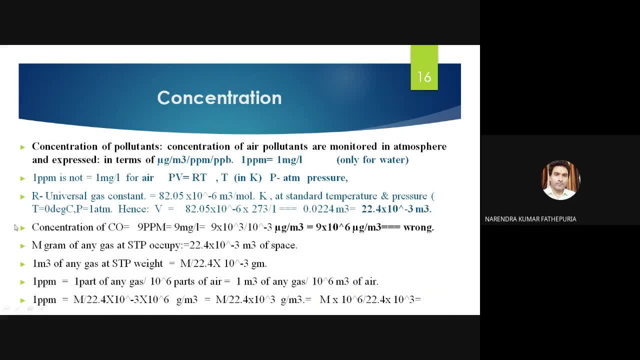 4 into 10 to the power minus 3 meter cube. you are getting it finally. Now you have to find out the concentration of carbon dioxide, carbon monoxide, sulfur dioxide, NOx. you can get it through this. Suppose concentration of carbon monoxide is given 9 ppm, 9 mg per liter, So 9 into 10 to the power 3. 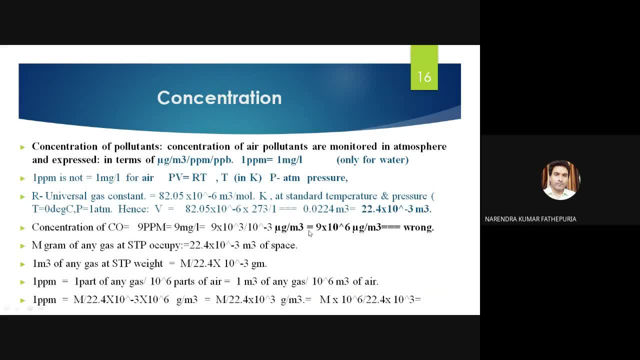 divided by 10 to the power minus 3, you will convert into the microgram per cubic meter. Liter to cubic meter conversion: you can do it based on this. you have to divide by 10 to the power minus 3, that you have done it. And mz to gram microgram, you have to convert it. 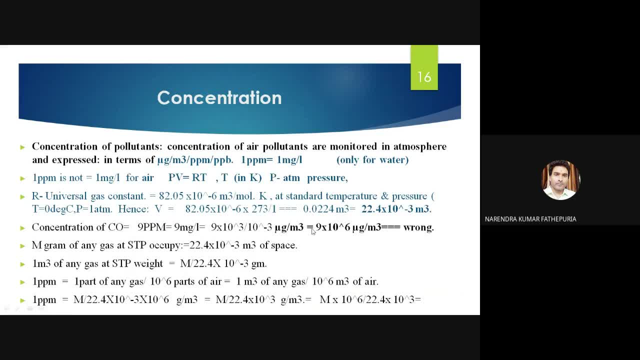 then you have to multiply by 10 to the power 3, that you have done it. then finally you got the unit here: microgram per cubic meter. So 9 into 10 to the power 6, microgram per cubic meter. you. 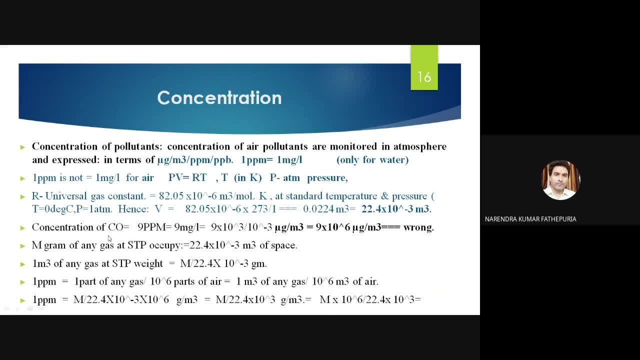 will be getting here. But this is not right in case of gases, right? So generally we do this calculation right: mg per liter we convert into in that case. but it is not valid for the for the gases case. For the gases case we have to go for the different. 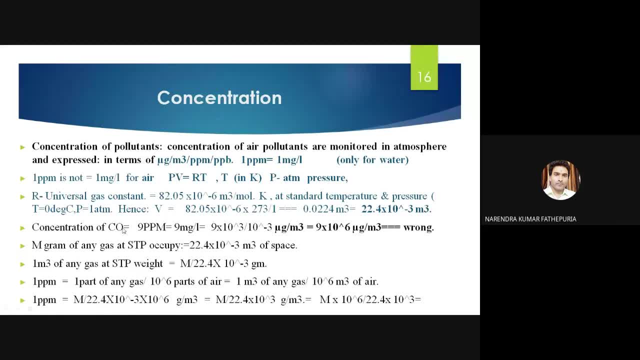 different gases. So for the gases case we have to go for the different, because liquid gases respire Generally. if you are getting an IMP thing, you will be directly converting micrograms per cubic meter, but it is not right. So here for the gases. 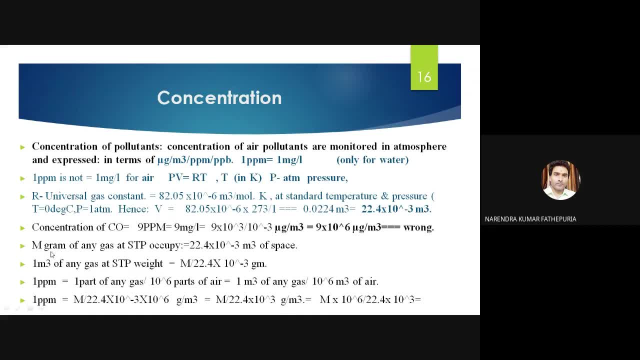 concentration. for measuring the gases concentration, the m gram of any gas at STP standard temperature influencer occupy as 22.4 into 10 to the power minus 3 cubic meter of space, as we have told here that we have calculated right. So m gram of any gas as STP occupy 22.4 into 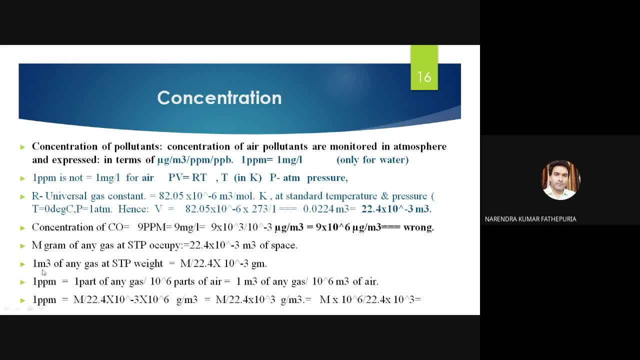 10 to the power, minus 3 cubic meter of space, Now 1 cubic meter of any gas at STP weight. you have to calculate m gram that you have taken. it divide by 22.4 into 10 to the power. 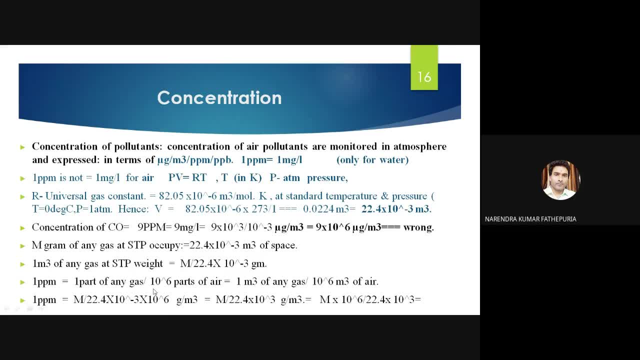 minus 3 gram. So 1 ppm is equal to 1 part of any gas. divide by 10, to the power 6 of part 10 to the power 6 part of air is equal to 1 cubic meter of any gas divide by 10. 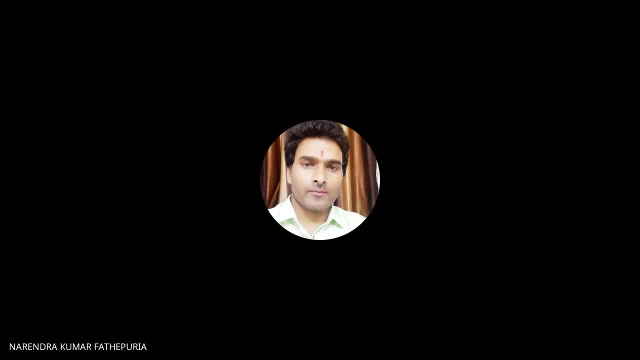 to the power: 6 cubic meter of air. So 1 ppm will be equal to Here m divided by 22.4,. I am doing a basic calculation here. 1 ppm will be equal to m divided by 22.4. into 10, to the power minus 3, into 10. to the power 6 gram per cubic meter. 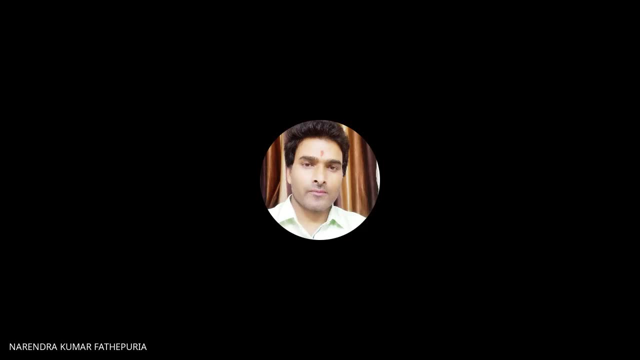 So you convert, finally, m by 22.4 into 10 to the power 3 gram per cubic meter. You can convert in microgram per cubic meter. you can convert in that way, So m into 10 to the power 6, divided by 22.4 into 10 to the power 3.. So if you want to convert a carbon, 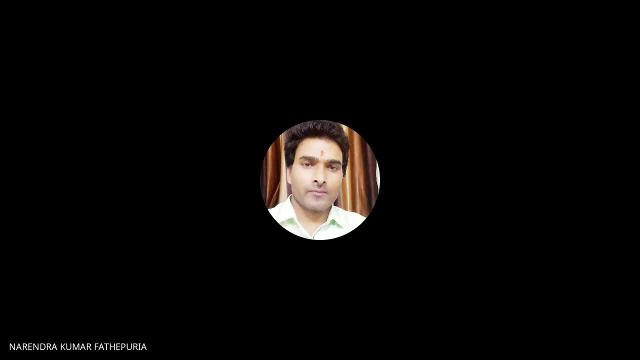 monoxide. the concentration of carbon monoxide is 10 to the power 6.. So you have to convert, you want to determine, you have to use this formula. finally, So at 1 ppm, at STB standard temperature and pressure at 1 ppm will be equal to this value will be given m gram. 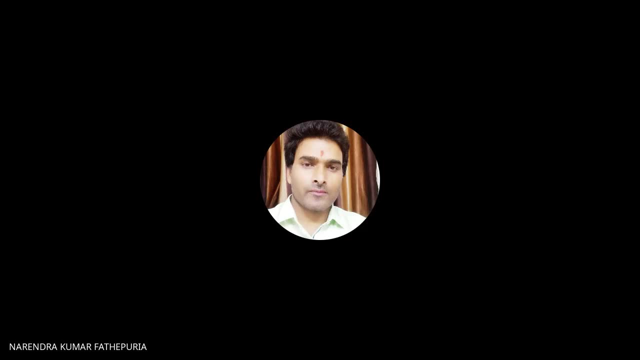 of a particular gas divided by. you have to divide by 22.4 into 10, to the 3 microgram per cubic meter. So this is the right estimation for it. Suppose, if you want to find out the concentration of carbon monoxide you have to go in that formula. So m is given as 9. 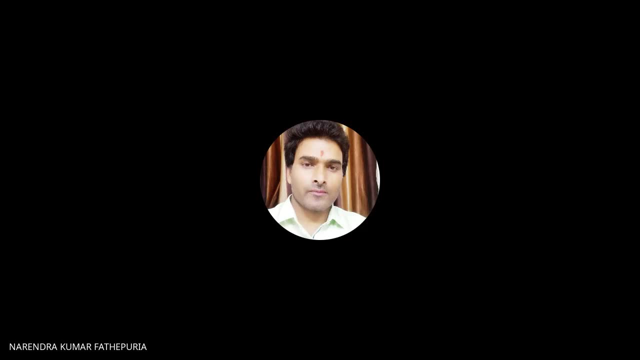 ppm, 9 mc per liter, respective conversion you have to do in that formula. And another thing: if you go reverse- 1 microgram per cubic meter at STB- then you have to. this will this equation. you will take it if you want 1 gram, 1 microgram per cubic meter. 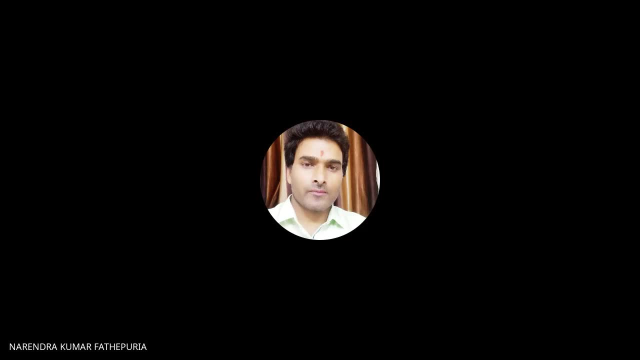 then it will be diverse here, 22.4 divided by m into 10, to the 4,, 3 ppm. So that also you can do So any of the conversion you can do. this is the right estimation for it, So that also you can do So any of the conversion. 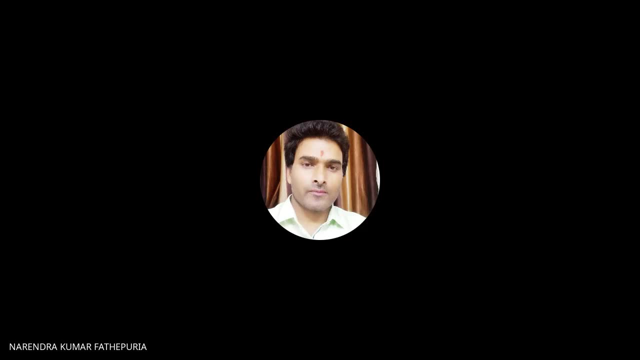 you can do So, any of the conversion you can do. this is the right conversion for converting up, for getting the concentration of particular gas. Okay, Generally, microgram per cubic meter. you have to take it everything. So 1 microgram per cubic meter will be equal to 22.4 divided. 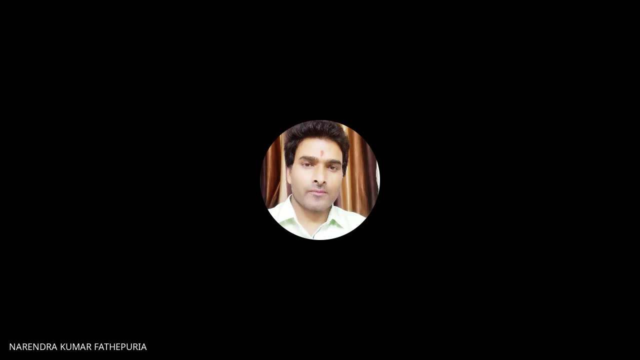 by m concentration is given there, multiplied by 10 to the 3 ppm mc per liter, you have to do the respective conversion. So 1 ppm at a respective temperature and pressure will be equal to given m gram. whatever the concentration is given ppm, whatever it is given m divided, 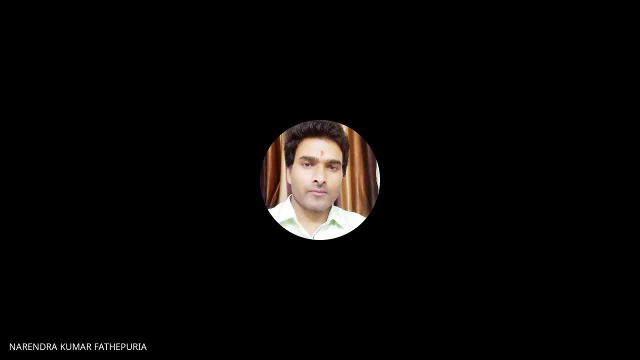 by m into 10 to the 4, 3 ppm. So 1 microgram per cubic meter will be equal to 22.4, constant multiplied with 10 to the power 3, this is constant 22.4. and to multiply with 10 to the: 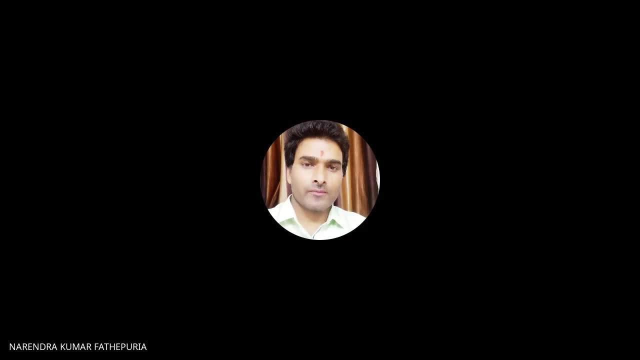 power 3, microgram per cubic meter. m is the molecular weight of the gas, So carbon monoxide molecular weight- you can take it 16 plus carbon molecular weight is now So 1 microgram per cubic meter at standard temperature and pressure will be the constant divided by m. 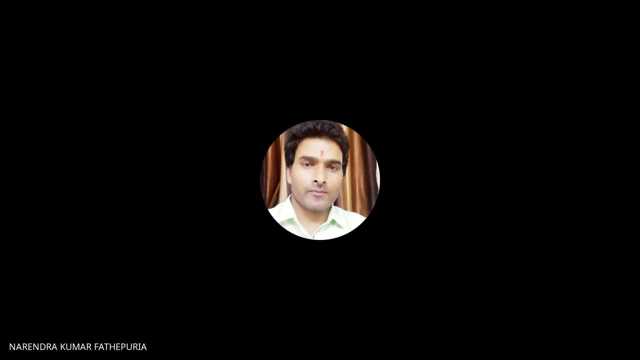 into 10 to the power 3 ppm. So these are the two formula: one formula, one formula and second formula. Same as it is. if it is a one path per billion at standard temperature and pressure, that will be the same formula. for it, the constant will be 22.4.. So this: 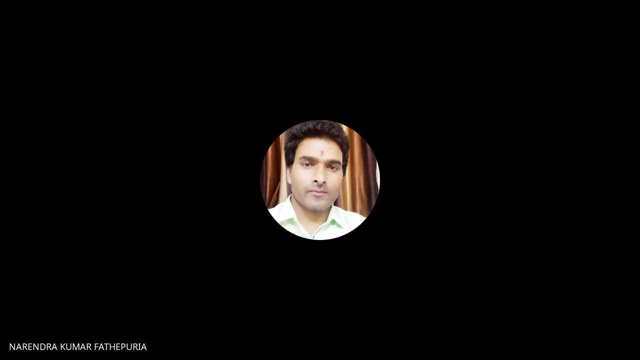 is the question now. the 9 ppm of carbon monoxide at a standard temperature or pressure will be 9 ppm. it is given into: multiplied with m molecular weight, divided by 22.4 into 10 to the power: 3 microgram per cubic meter. 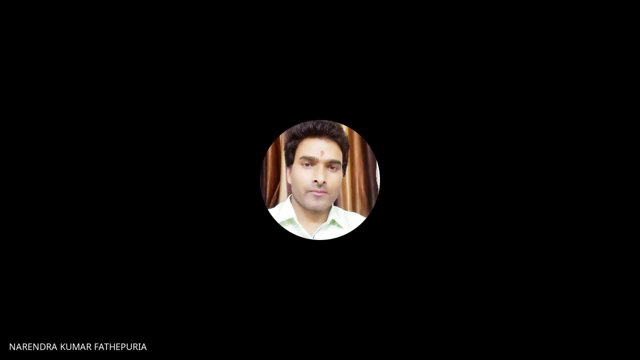 Into what is the molecular weight of carbon, molecular weight of oxygen, addition of both two, So molecular weight 9 into carbon, 12 plus 60 divided by 22.4 into 10 to the power 3, this is the right estimation, So you will. 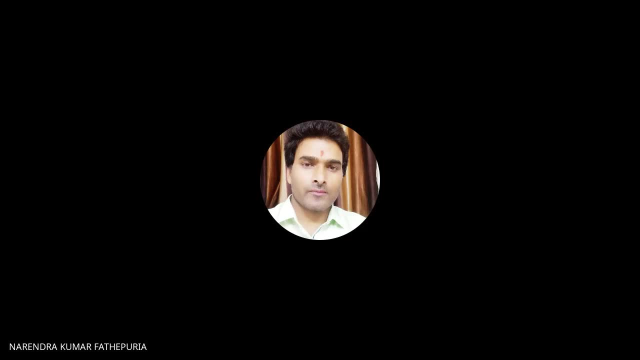 be getting at 11,250 microgram per cubic meter of concentration in the atmosphere. Like this you can measure the gas's concentration into the atmosphere CAMتmm. so it will be 12, 11.25 mg per cubic meter CAMtmm. it is needed for its concentration So you can match this. 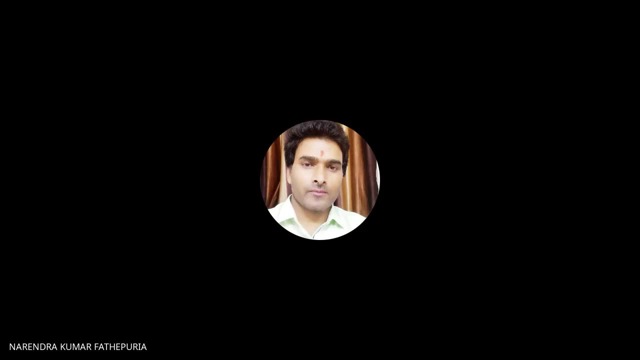 same if the gas. it isiso 108, where g is poetry. from current temperature into current cubic meter: 11.25 mc per cubic meter. you will be getting here correct. now the concentration of chloro. second question: concentration of chloroform. you want the same way, you can do. 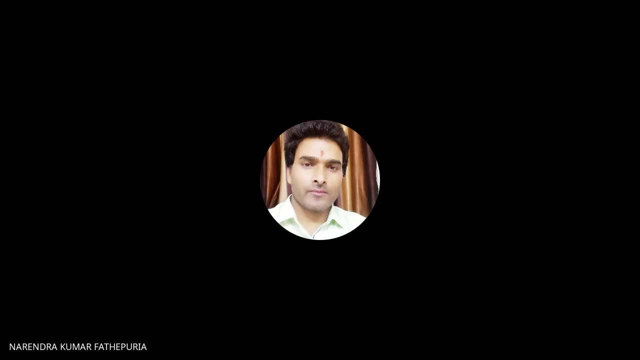 it like this: also: one microgram per cubic meter. it is given in 0.4 microgram per cubic meter. now the second equation you have to use, this is the given here. one microgram per cubic meter is equal to: this is your, this is your um formula, constant divided by m in ppb. so 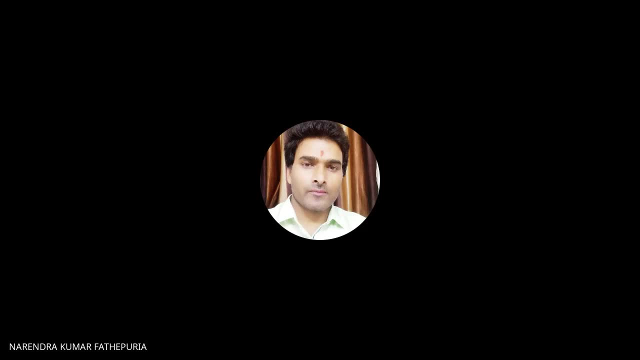 the constant will be equal to 0.08205. into 293, 293 is in the temperature. divided by one, you will get it as 24.04. the 0.0822 a2 uh- this one, 8205- is the molecular weight of this chcl3. 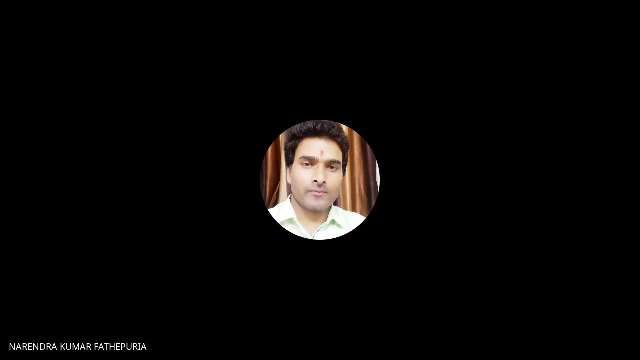 so 0.04 microgram per cubic meter will be equal to here: see, this is the avogadro constant: r you have measured. no, this one is the avogadro constant. i will show you here. here we have done. no, here, this one we you have calculated, and this one was the complete 24.4. 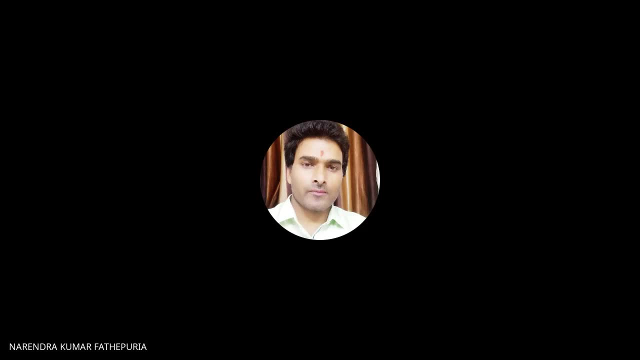 cubic meter: same. this is the 24.04, 24 point. yeah, because here, uh, here are 293 into 23 divided by 1, so 24, 24.04. you got it. now you can apply this formula here also, then you will get it finally 0.08 ppb. so like this you have to measure the. 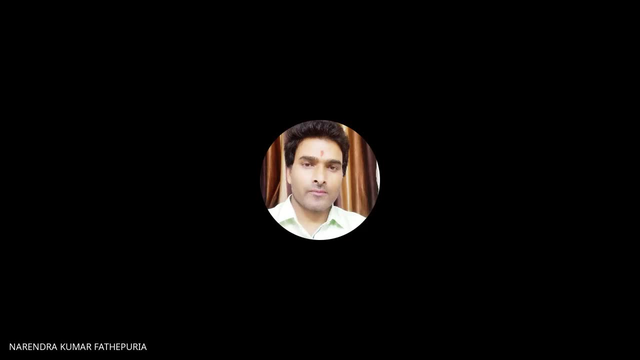 concentration of various gases in a atmosphere. now next question is: convert 120 microgram per cubic meter of so2 into ppm and ppb at. temperature is given at 10 degree celsius and pressure is 1. atmosphere sulfur molecular weight 32. there is a oxygen of 16 there. i can't give English, so it's. 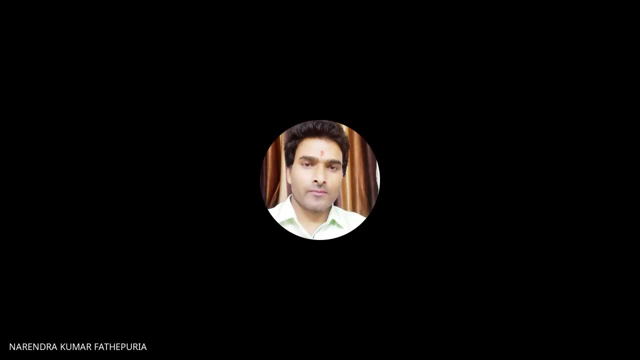 system. it is not given. you keep always remember the the table. no, gas is stable. so this is the formula one: microgram per cubic meter is equal to constant divided by m, so you can write it: 23.22 through the gas constant. you have measured with this 1. 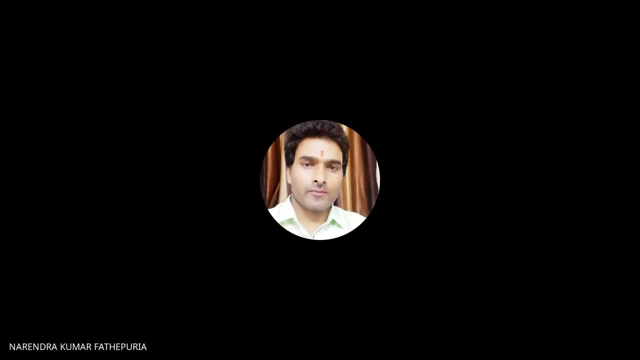 equal to 32, so you will be getting at 0.362 b 28 ssd. is the ppt visible? yes, oh, disconnected. Just a second. Please let me know if anybody is not busy, because I'm busy in explaining that From how long, like how much, before it disappeared? 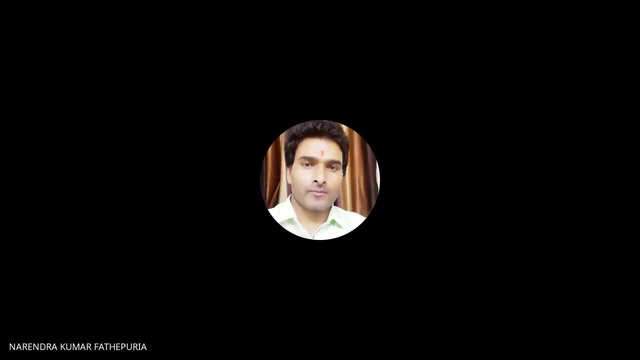 Five minutes, Five minutes only This net can be set here. Just a second Five minutes. What is in the net? One minute just. internet problem is there? Okay, All right, Okay, All right. Okay, All right, All right. 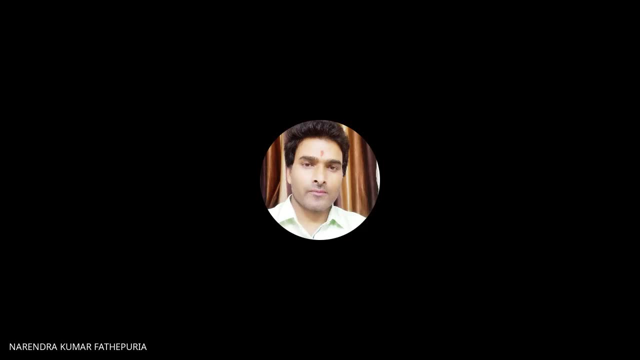